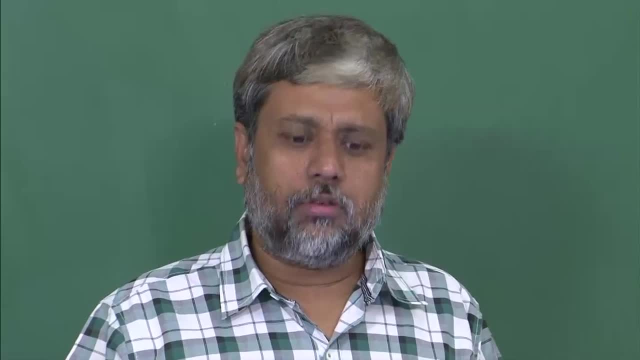 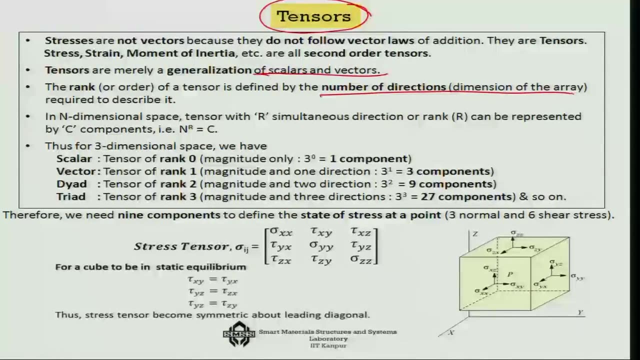 that how scalars and vectors could be. special case of tensors of certain ranks. The rank of a tensor is defined by the number of directions or dimension of the array, that is, the number that is required to describe it. So suppose we are talking of an n-dimensional space. 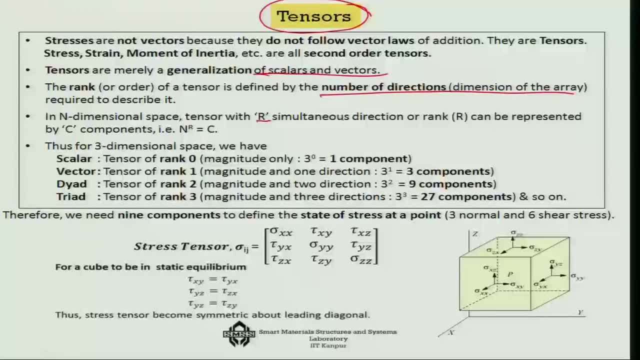 and we are talking of a tensor with r direction or rank r, then it can be represented by c components, such that n to the power, r equals to c. Now let us try to use this in terms of our day-to-day experience. Suppose we talk of a scalar quantity. that means say how. 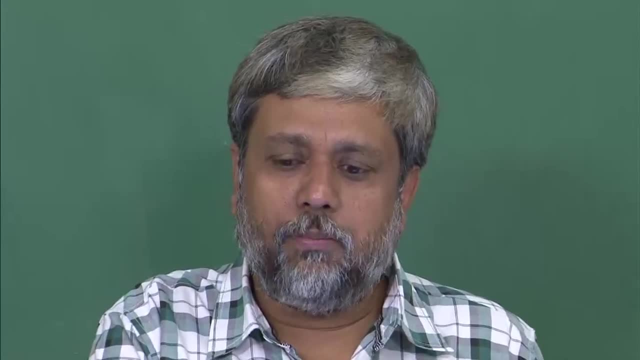 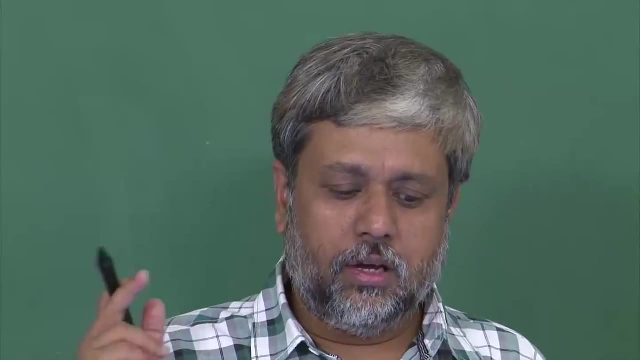 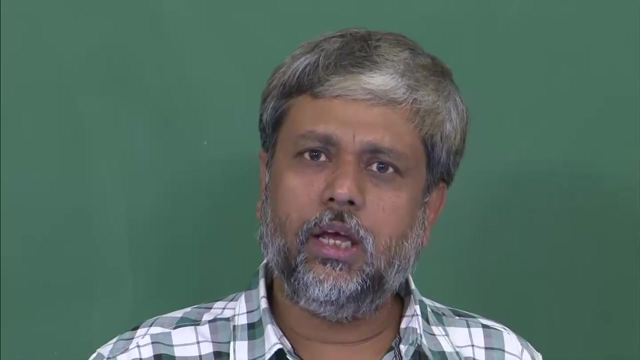 many pains. you ask me, how many pains do I have in my pocket? So suppose if I have one pain in my pocket, then this is a scalar quantity, and this scalar quantity can be considered to be a tensor of rank 0 in a three-dimensional space. In other words, n is here, 3,, r is here. 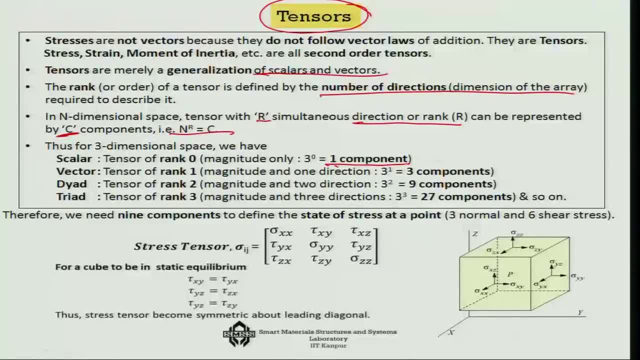 0, and hence 3 to the power 0,. that is only one component without any sense of direction. The number of pains, that is only the number itself. that is a scalar quantity. Now suppose we talk about that. how do we move from a position a and to a position b? So now I do not only 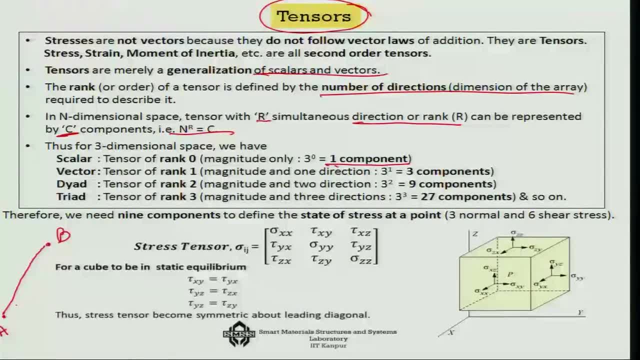 need the distance to cover, but also I need to say that which direction I will be covering. So, for example, you have to go this way. So it was presented this way, the combination of directions in order to reach this location. 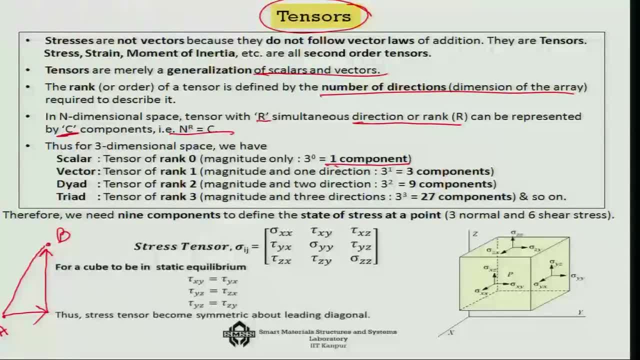 So if you have this kind of a sense of direction, that means you have a magnitude as well as the direction that is associated. so it is 3 to the power, 1.. Now, in a three-dimensional space that means you need three components, and you know, wonder that any vector in a 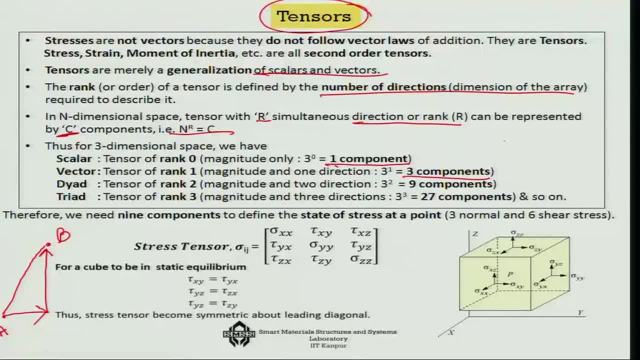 three-dimensional space. you always denote it with respect to 3 unit vectors, if you remember: i, j and tw Channel and k, So that you can actually say that this distance d is nothing but something like x, i, y, j and z, k. So that is how you define the you know vector in terms of the distance. 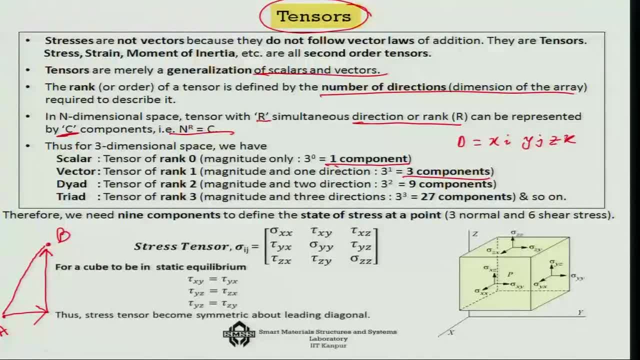 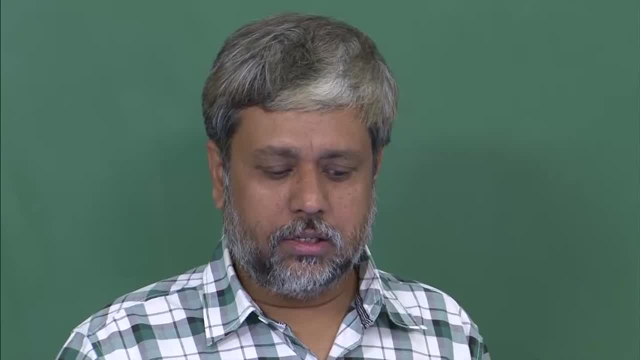 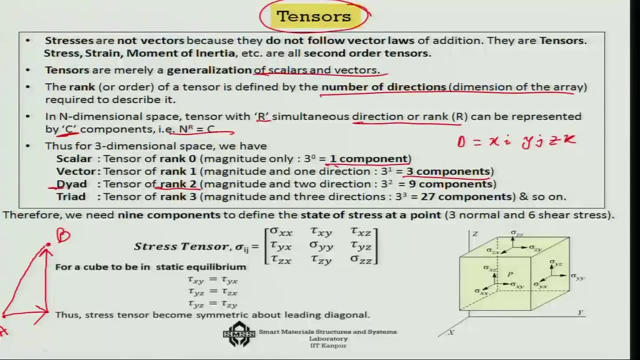 of velocities, etcetera. There are many such things where these you know. first, rank of tensor is important. When we will talk about stress, the stress is actually a something which is of rank two. So it is a tensor of rank two, which is also known as a dyad. So 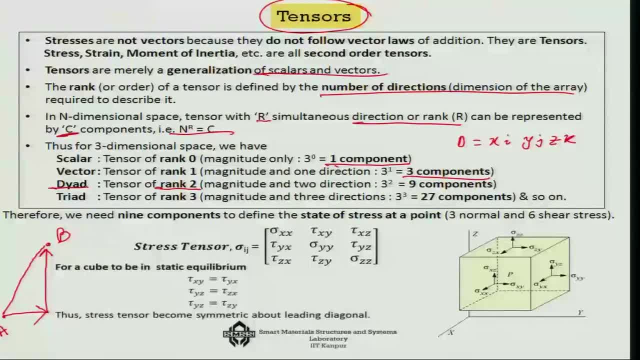 that means here you need a magnitude as well as two directions. every time That means it is three square, or in other words, nine components are needed in order to define the stress at a point. So that is why I told you earlier that just a very simple generalization of a stress, as 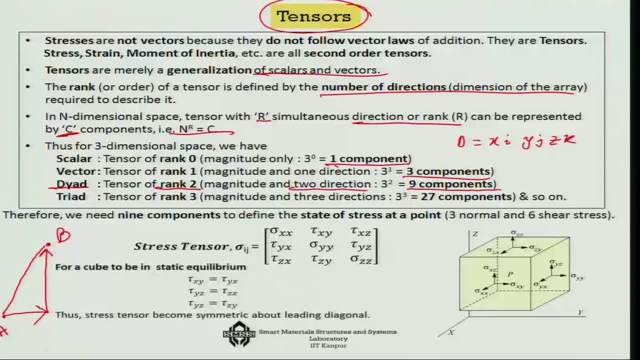 a force per unit area does not really make a sense, because which area are we talking about? Now you have a much better definition of stress. that suppose you consider a point and you have a. you consider a cube all around this point. That is what we are showing here. 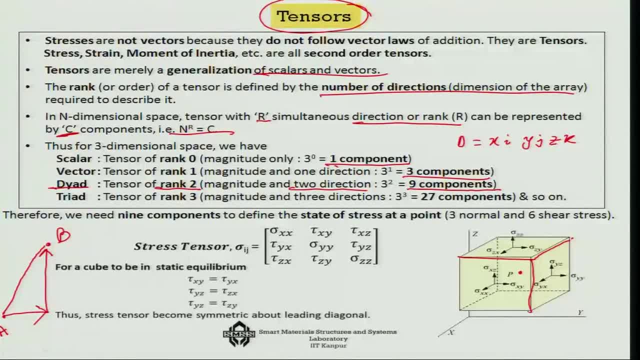 right, a cube all around this point. Then you have a field condenser, one inside and one outside. this is actually a composite, Freddy. another zone, right? So this one is actually a composite, eh. And then another zone. we have such like a. 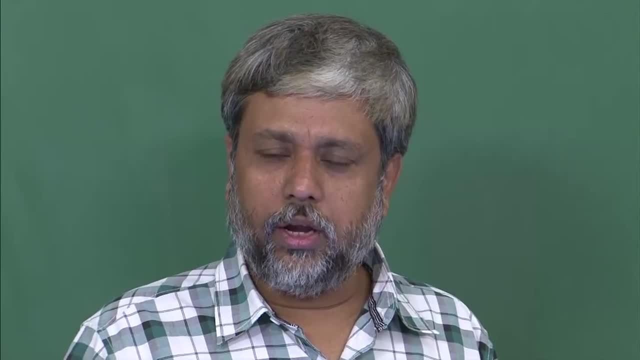 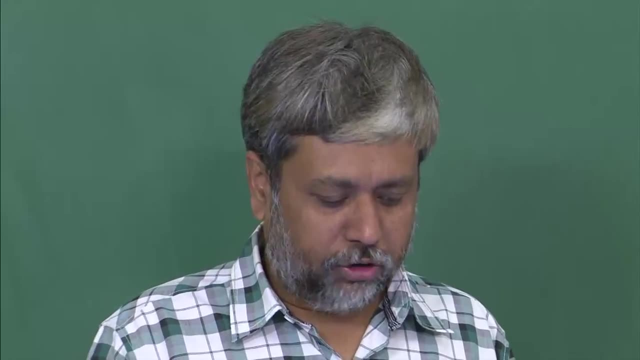 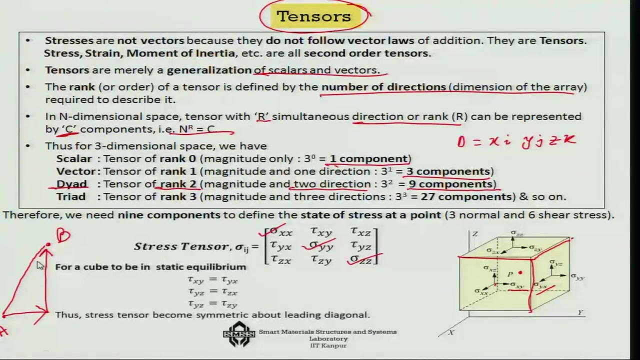 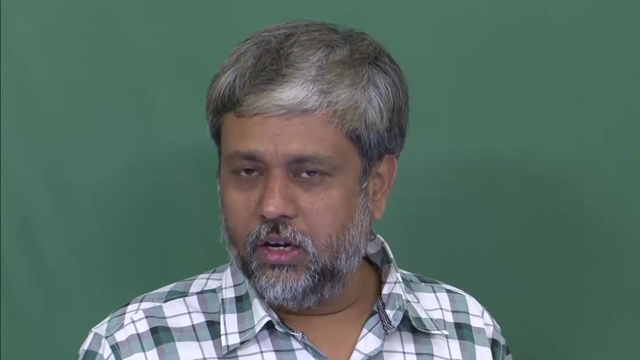 D attack, where- which is different- rank two tensor. Similarly, strain is also exactly the same way- tensor of rank two. So you need two rank two tensors to define the stress and the strain. Naturally, if you are talking about modulus of elasticity, then actually you need a rank four in order to 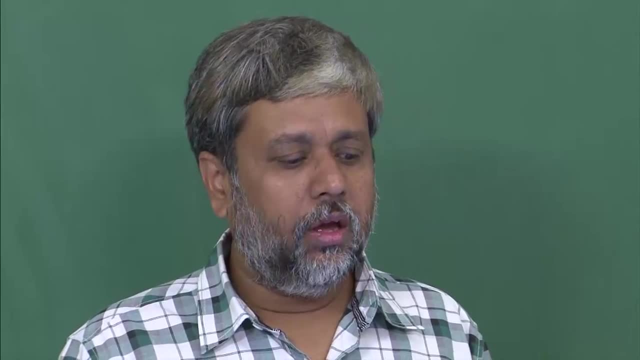 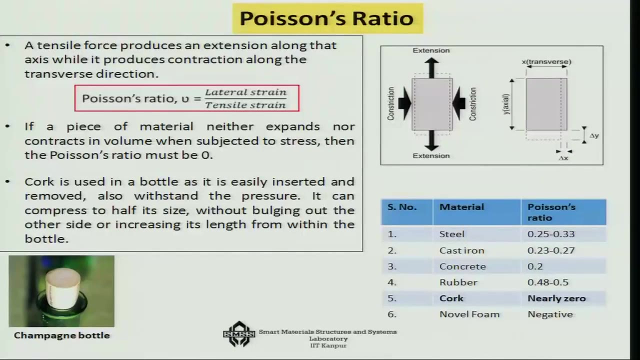 define the relationship between the two diodes. Now there is something more, So that is about the stress. The other interesting thing is the Poisson's ratio. This refers to that when I am actually extending a material. Let us just take this example that we are extending. 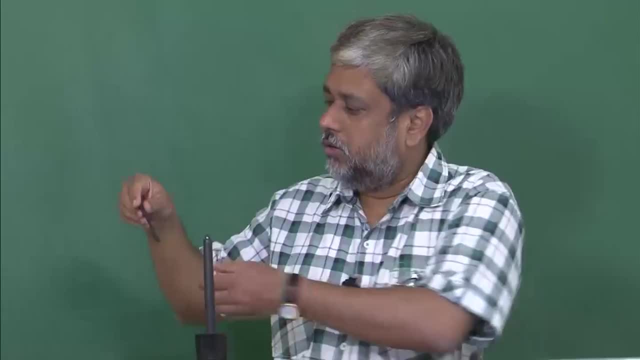 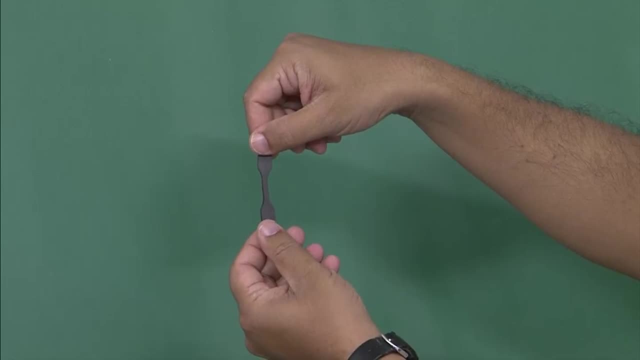 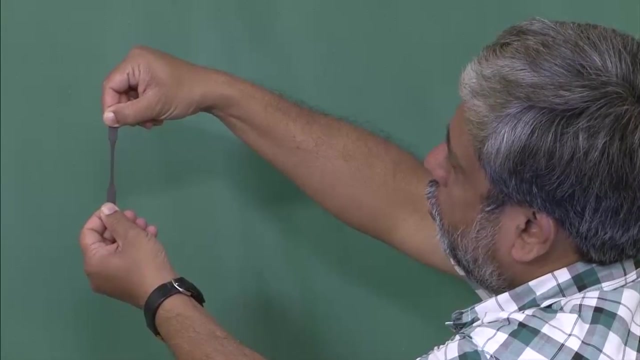 in a universal testing machine and I am applying the tensile force. this is a rubber sample and you can see that how the thickness is reducing in the other direction. so this being a rubbery material which has a Poisson's ratio close to 0.5, this shows beautifully. 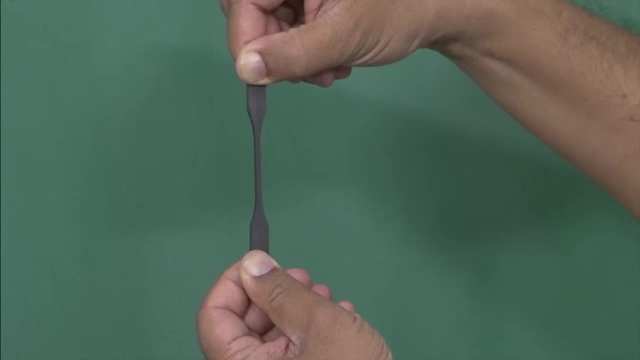 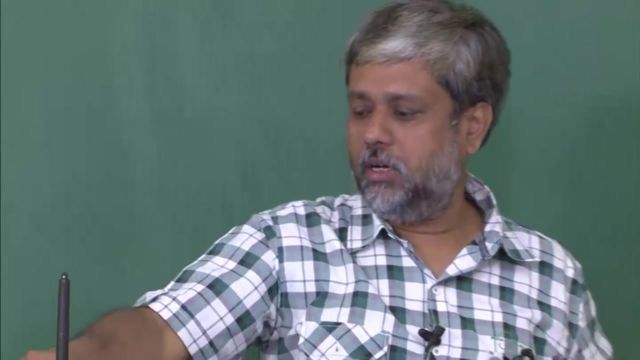 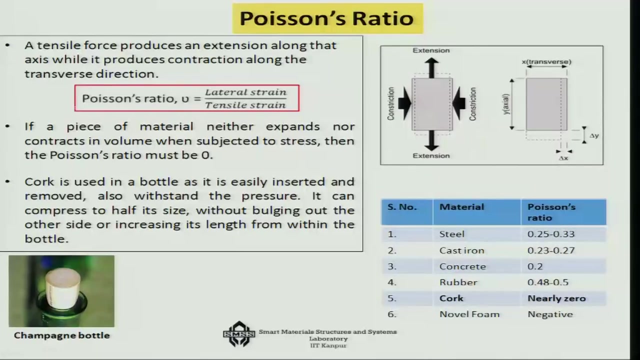 that how it is narrowing down in the direction perpendicular to the application of the force. so this, you know, nature of a material is actually depicted by what we call the Poisson's ratio of the material. so that is the Poisson's ratio, which is the ratio of the lateral strength. 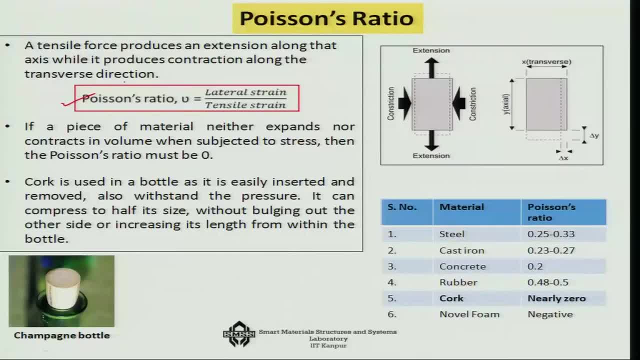 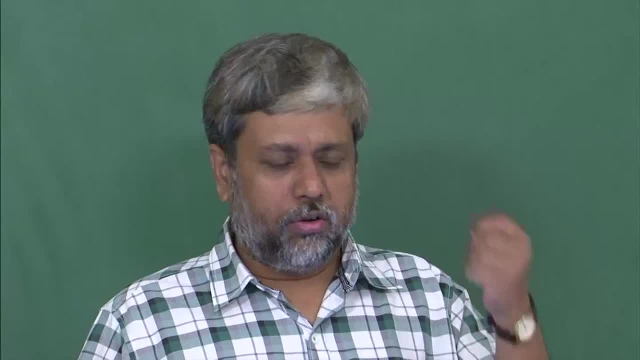 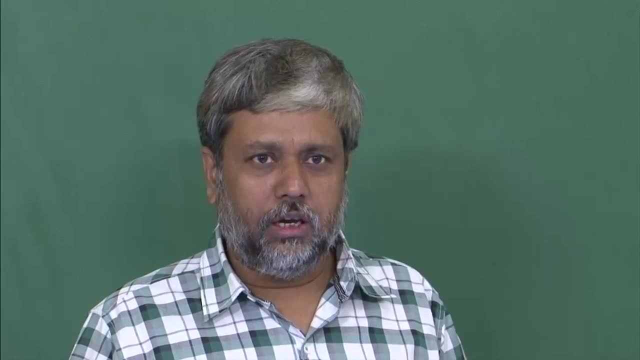 to the tensile strength. now, if a material does not exhibit this behavior, there are some materials which does not exhibit this behavior. for example, a bottle. in a cork of a bottle, they generally neither expand, you know in terms of when you are compressing it, or not the other way round. So they have. 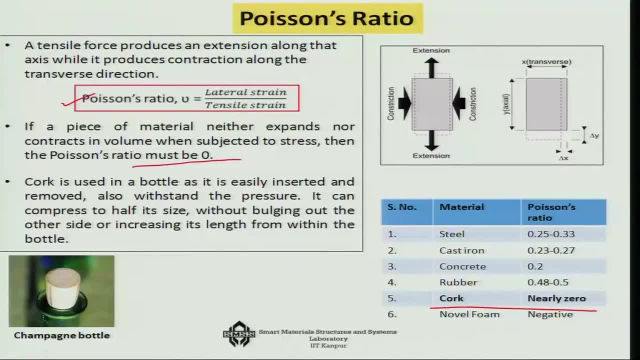 a Poisson's ratio which is close to 0. In fact, cork's Poisson's ratio is nearly close to 0.. Most of the other materials in the day to day experience that you use, for example the metals, they have a Poisson's ratio. 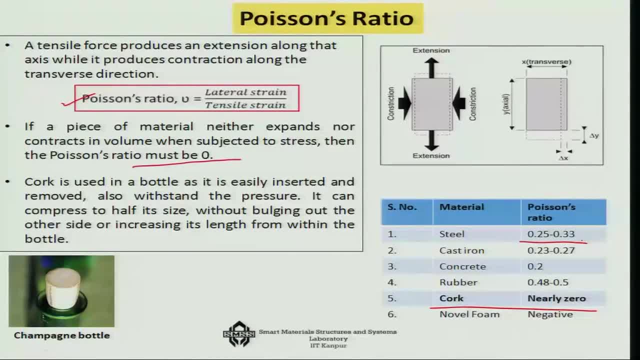 between 0.25 to 0.3, etcetera. Concrete has a Poisson's ratio of 0.2 and rubber has a Poisson's ratio, as I have just now shown you, and that has a Poisson's ratio close. 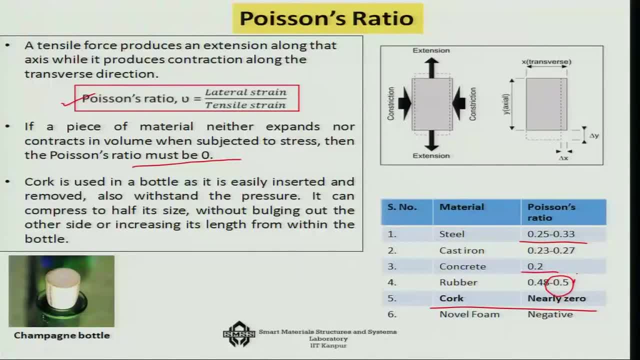 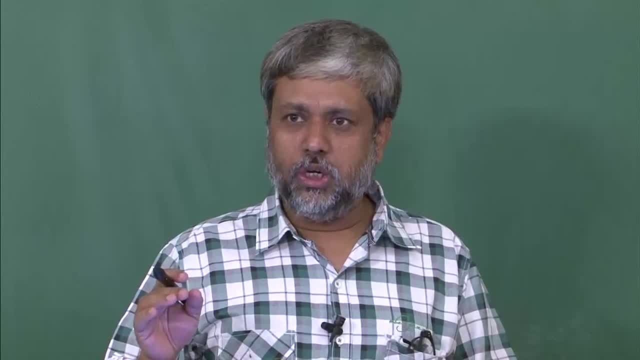 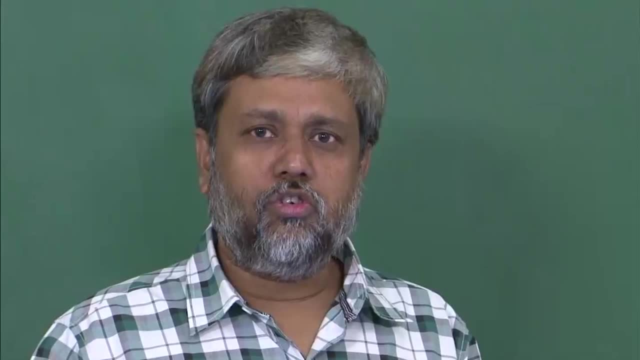 to 0.5.. Can a material have a negative Poisson's ratio? That means when we are actually contracting the material or expanding the material, let us say, just like that rubber experience, when you are expanding the material Instead of contracting, can it expand on the other direction? 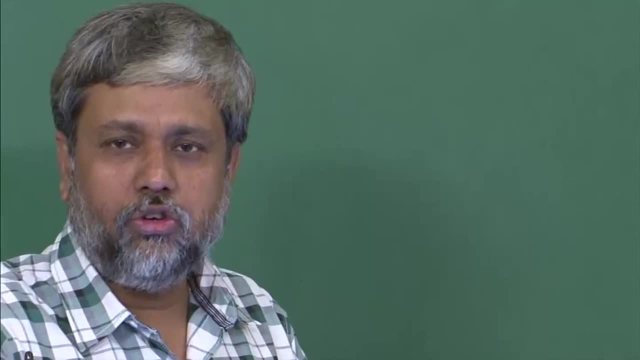 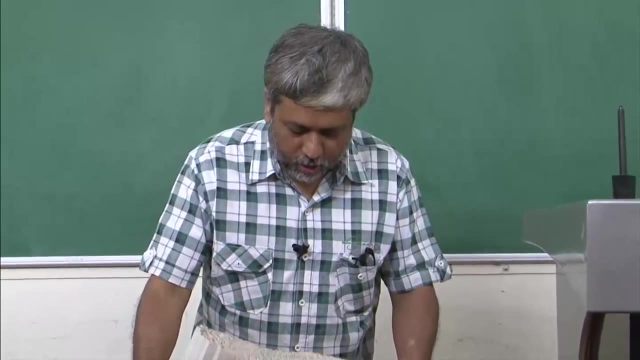 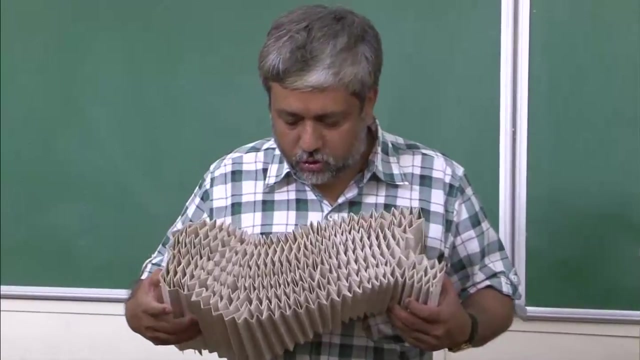 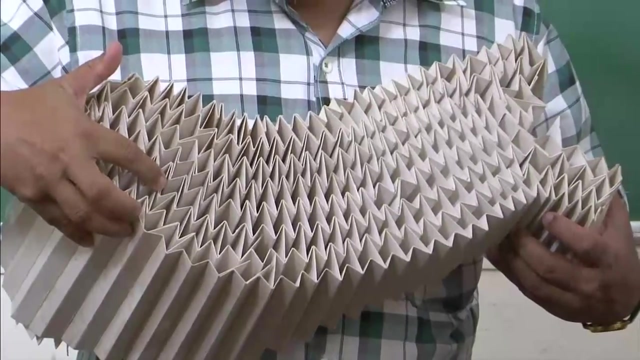 Yes, in certain cases it can. Let me just show it to you through an example. Now, this is actually a, you know, a kind of a reentrant honeycomb structure. This is a. this is a auxetic structure. So in this auxetic structure, if you look at it, that it is the each of the honeycombs instead, 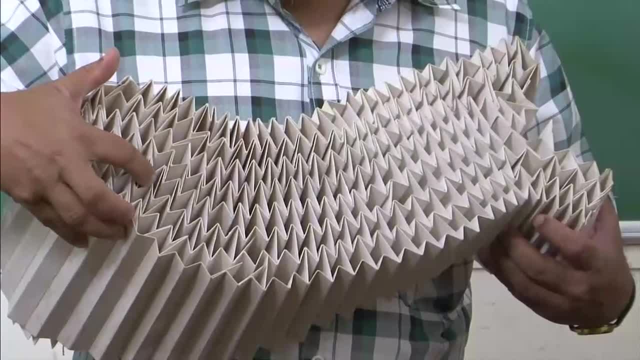 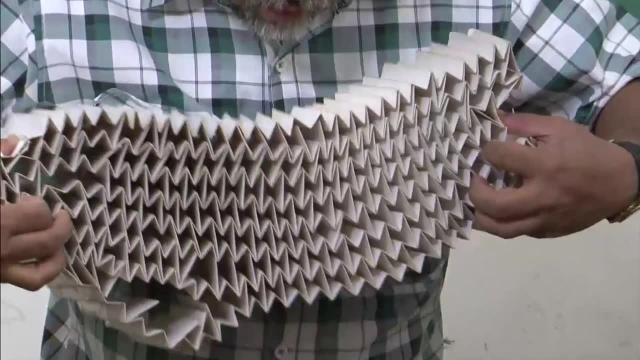 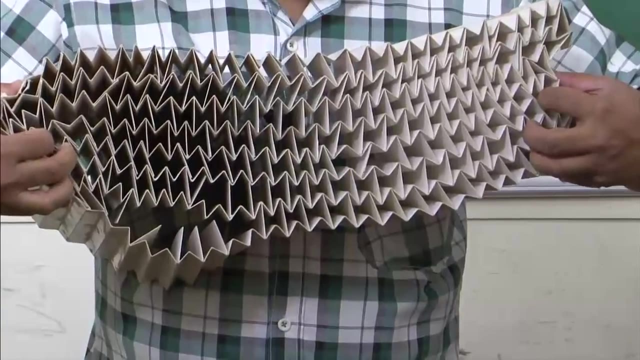 of the honeycomb with a positive angle. they are having a negative angle, each one of them And these. what happens in such a case? suppose? now I am trying to expand the material, So I am expanding it in this direction. You see that, the other direction, that is in the perpendicular- 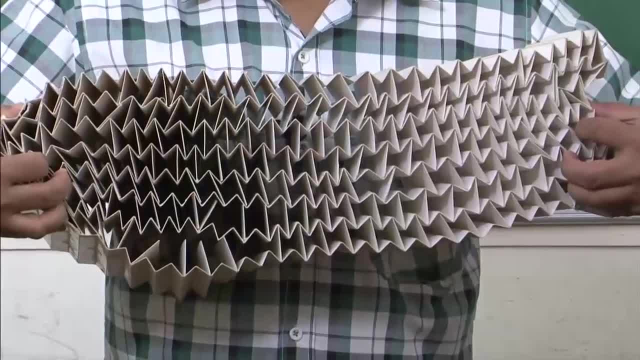 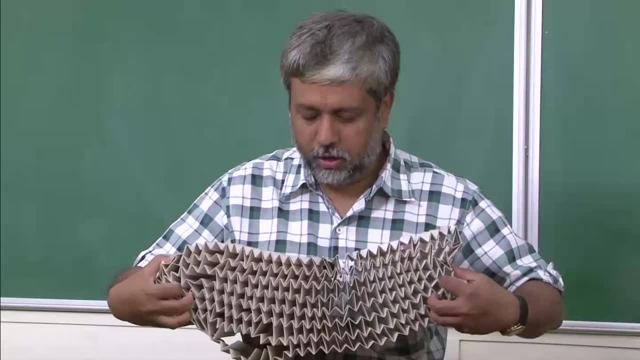 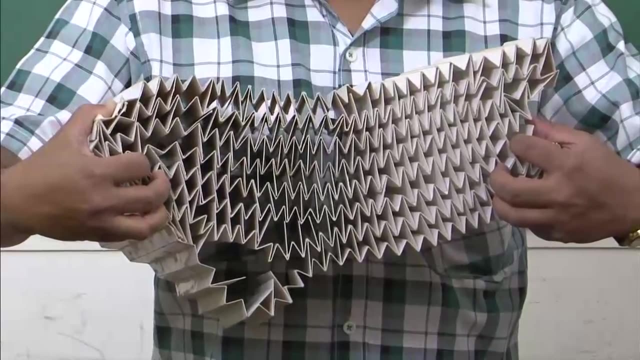 direction. instead of contracting, it is actually expanding The more these reentrant angles are actually unfolding. it is expanding more and more So, and the other way, when I am compressing, you can see other directions. instead of expanding, it is also getting contracted in the other direction. So expansion is creating. 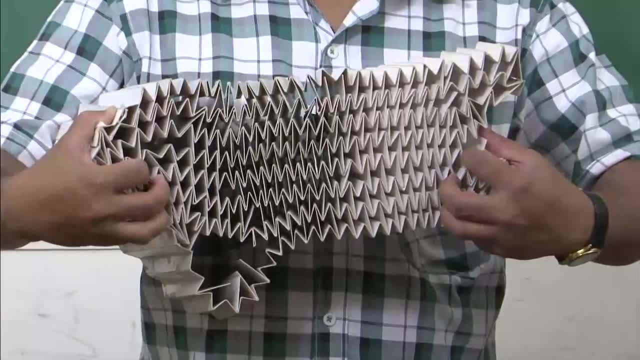 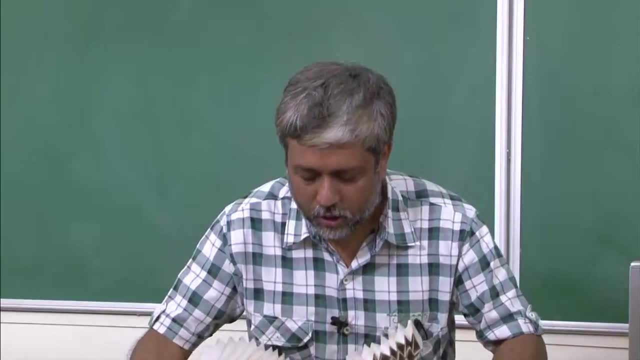 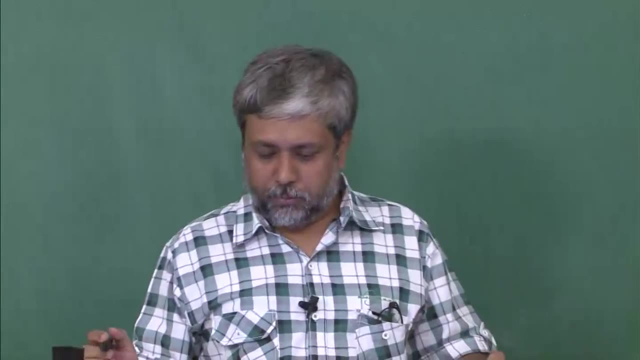 function. compression is creating compression. That is the beauty of an auxetic structure, of a structure which is having a negative Poisson's ratio. So we have talked about various types of Poisson's ratios and that definitely is a very important. 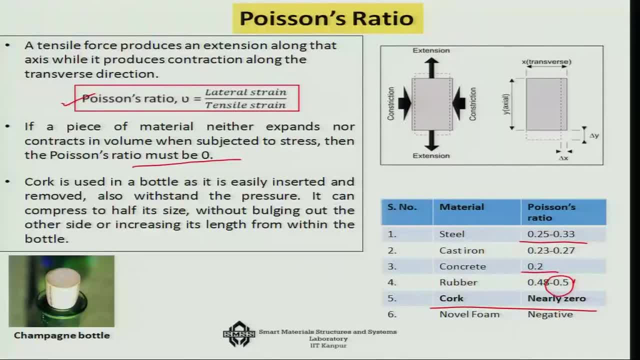 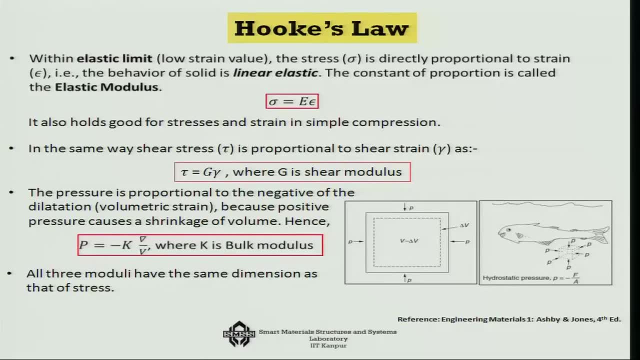 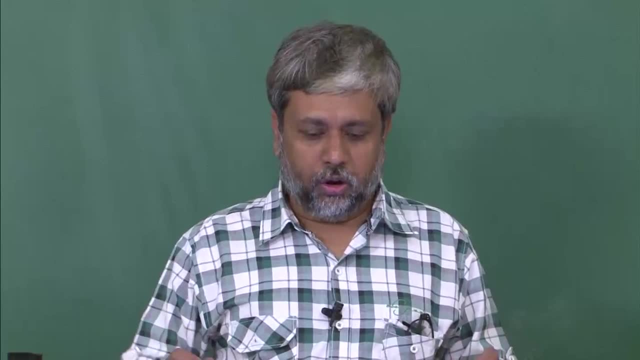 consideration, a material property consideration, when we are actually selecting a material. Now we also have talked about stress and strain. The stress and strain are related by something which is known as the Hooke's law. So there are, of course, the Hooke's law, which actually 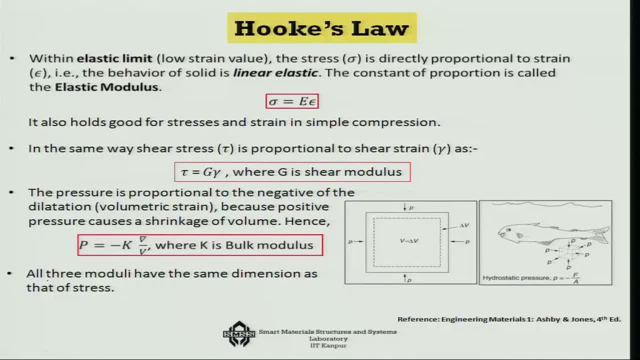 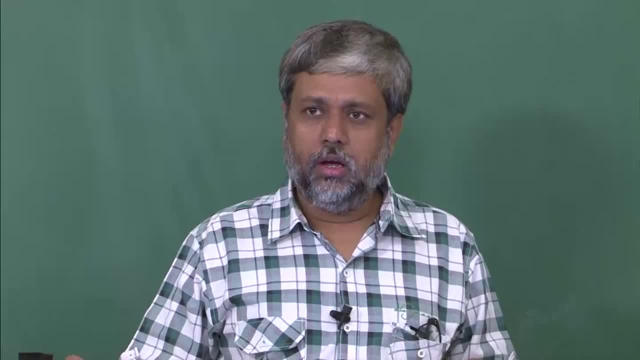 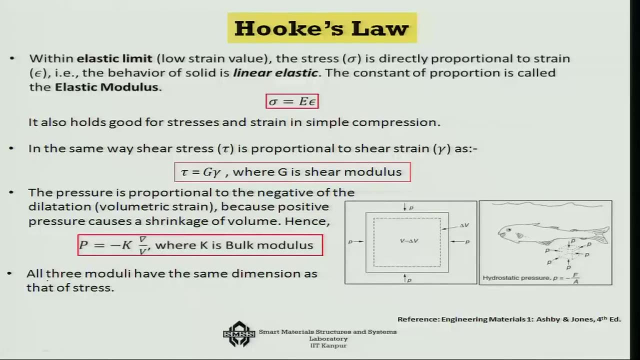 can be considered as a relationship between a single stress factor and a single strain or, in a generic sense, between a stress tensor and a strain tensor. So in that case, if I consider the relationship to be a matrix relationship, that means sigma i, j equals to. in that case it will be e i j k l, epsilon k l, So that 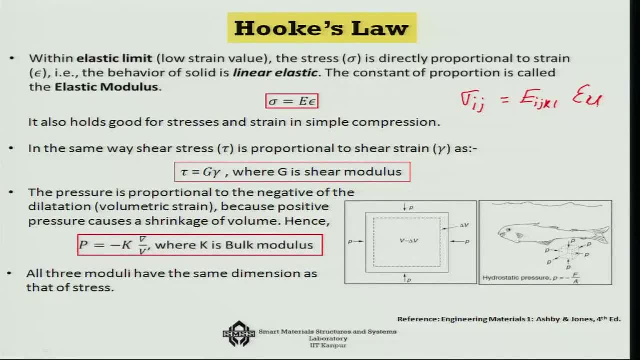 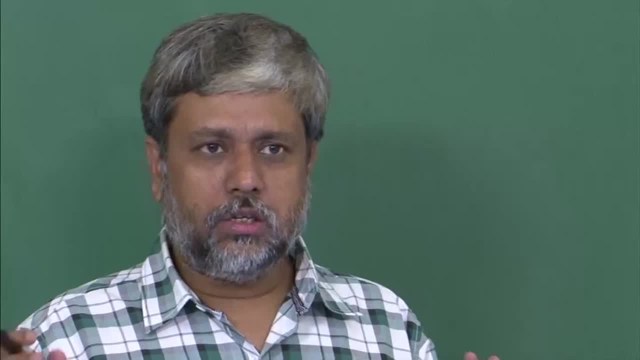 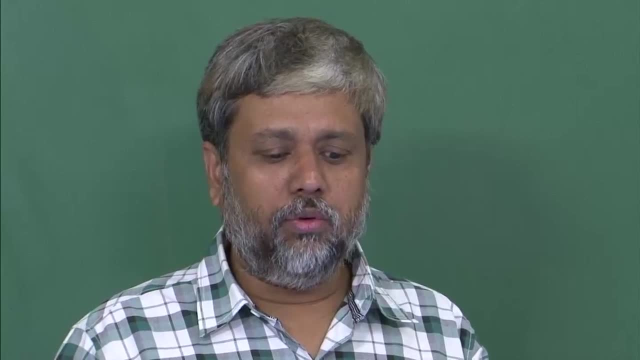 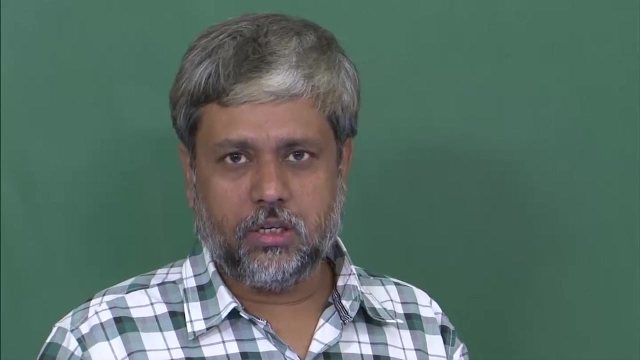 is the most generic Hooke's law. So basically, Hooke's law is something which is relating between the stress and strain, And each stress and component within a linear elastic domain is generally found out to be having a proportionality. That means if you increase the stress two times, the strain also will increase two times. 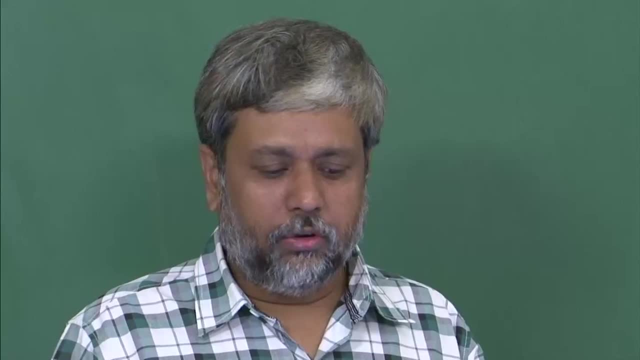 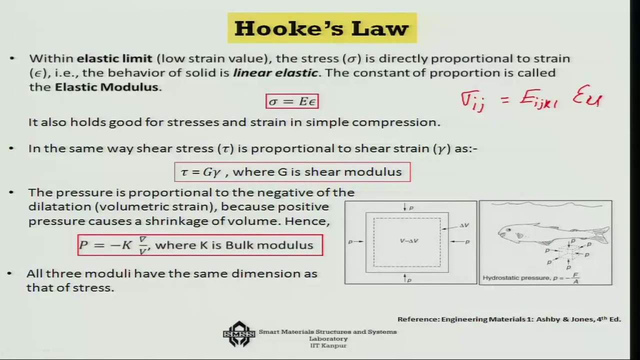 So there is a sense of proportionality that will be there between the two. So that is the simplest form of the Hooke's law which we also call. you know, the Hooke's law. So we also refer that if we do it for a component, then this, actually the e, becomes what we. 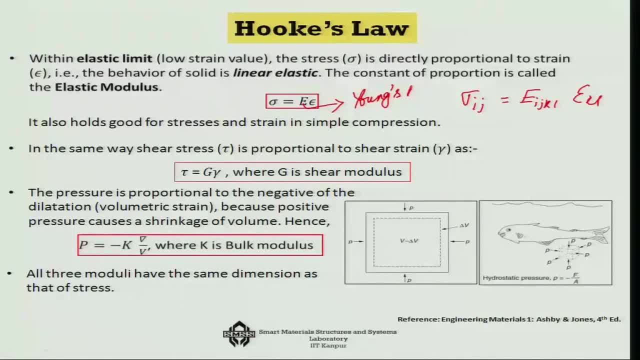 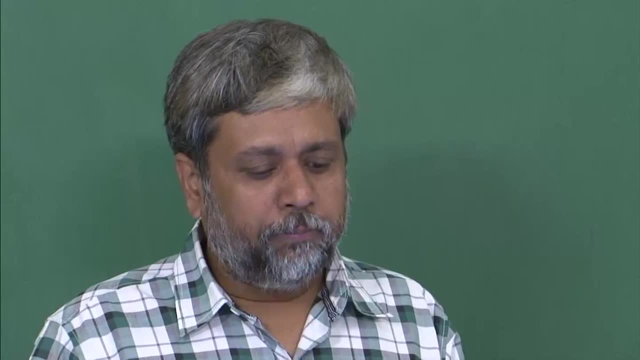 say, as the Young's modulus named after one of the most famous physicist and physician, Sir Thomas Young, who had first, you know, made very important notes on elastic behavior of materials. Now, the way a normal stress component is proportional to the stress component. 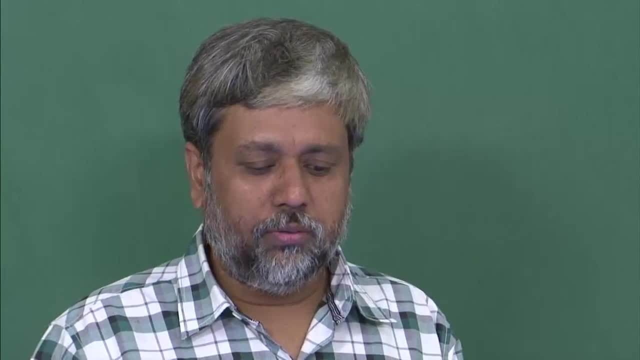 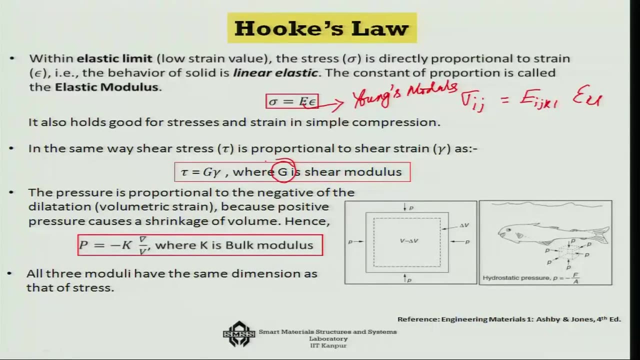 is due to strain component And related by Young's modulus. similarly, if you have a shear stress component, that will be proportional to shear strain And there the modulus of elasticity is referred as shear modulus or G, And if you remember the case of that, 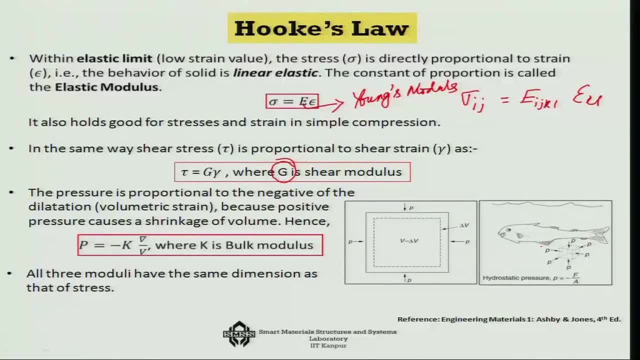 hydrostatic pressure case. there actually it is not happening the change in a direction, but in terms of the volume change. So you consider it for any fluidic case. so that's why the节dual rate changes directly, and then it becomes a stress component and the 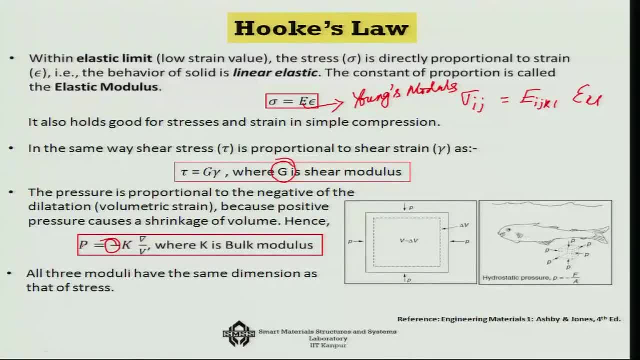 the negative sign is actually introduced here, because the positive pressure causes a shrinkage of volume. So here you get the volume change as the volumetric strain, and that is related with the hydrostatic pressure, and hence the modulus here is known as the. 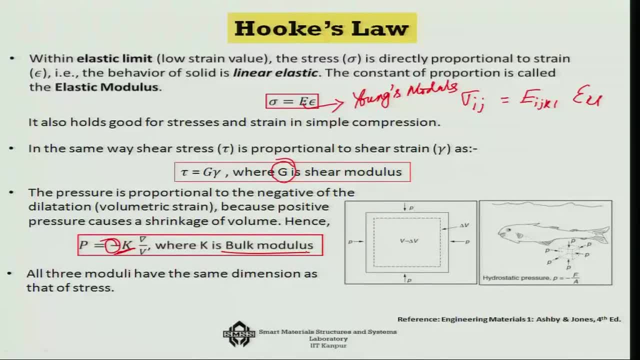 bulk modulus. So we have three different modulus: The elastic modulus- in the first case it is Young's modulus- shear modulus and bulk modulus. All three modulus, however, have the same unit in terms of the unit of the stress, because the strain is unit less. 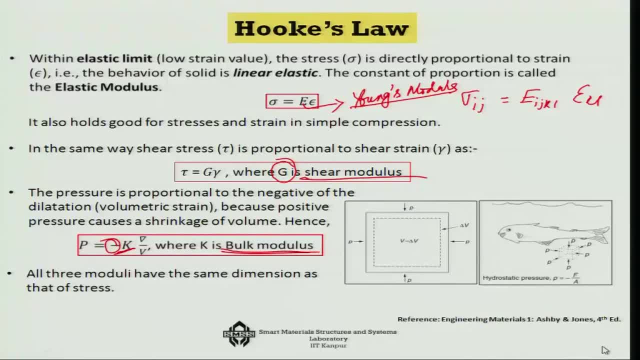 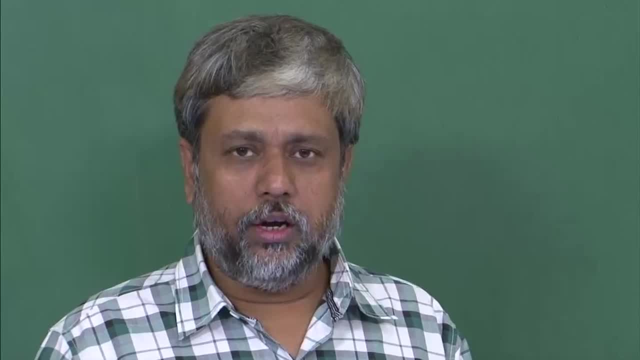 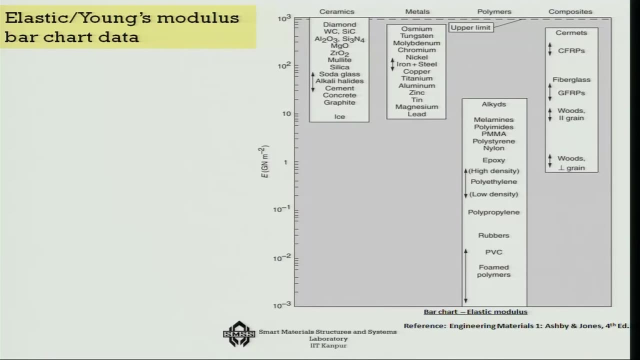 So it has the same unit as the unit of the stress. So that is about the Hooke's law which correlates between the two. So this is the stress and the strain and you can get actually the elastic modulus of the system. The point is that this elastic modulus varies and this is a measure of actually 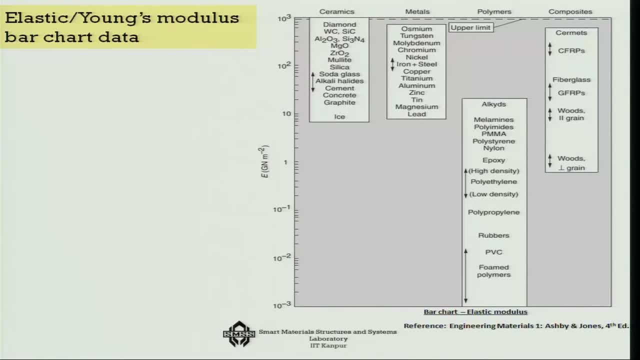 the stiffness of the system The way very easily. I worked with the rubber sample, with the steel sample- if you give me I may not be able to work so easily- So it has a higher stiffness, that means a higher modulus of elasticity. Now this is depicted in a beautiful 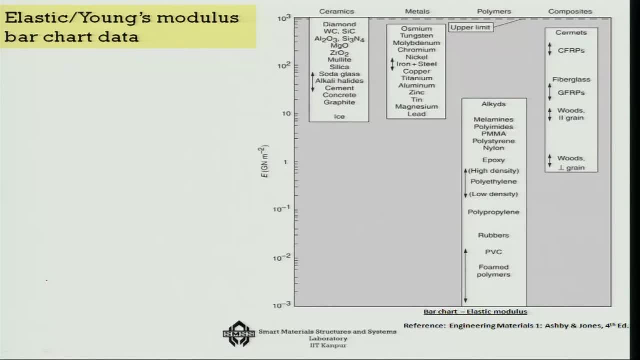 chart from actually S dish and Jones, and that he gives the elastic modulus for different groups of types of materials. For example, if you consider ceramics, they have generally a very high elastic modulus, like diamond, and then they may have some of the things which may have lower modulus of elasticity, something like say, for example: 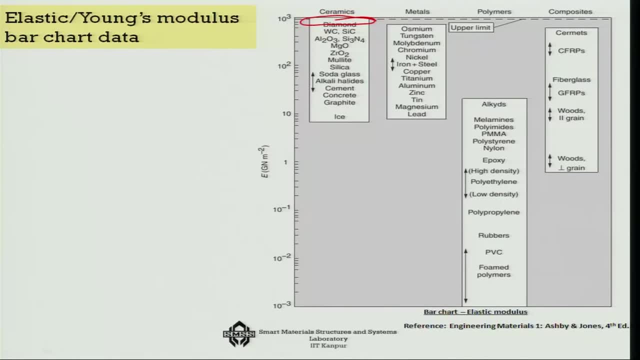 the glass area is down and it is purple and get very high. So these are the same Kerry's modulus. they have very good amount of elasticity. They are very high, less ef a FPS. Moreover, they have a very high modulus. you know, You do not control ang first, because they might. 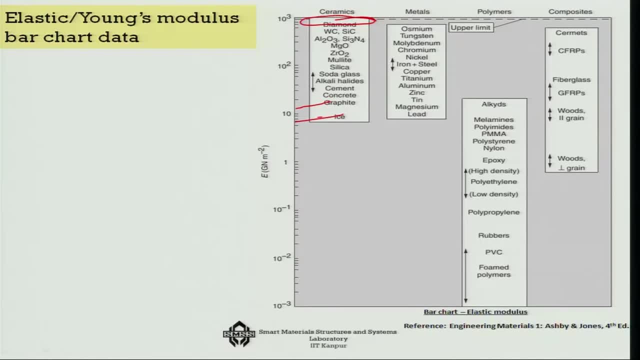 not have very high modulus, only on the right hand side only. But then they have these 好。 glasses, or the eyes, or the graphite, the cement. they may have somewhat lower modulus of elasticity, But in general ceramics have reasonably high modulus of elasticity. 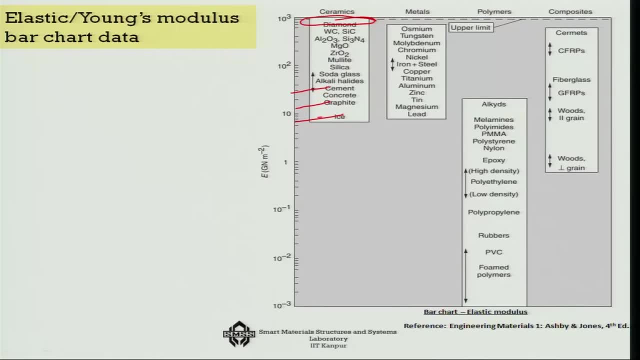 If you look at the metals, there are some metals which shows quite high modulus of elasticity. For example, tungsten is one of them. chromium is another of them, no matter. that is why, for the making the super alloys, this kind of materials are used, because they 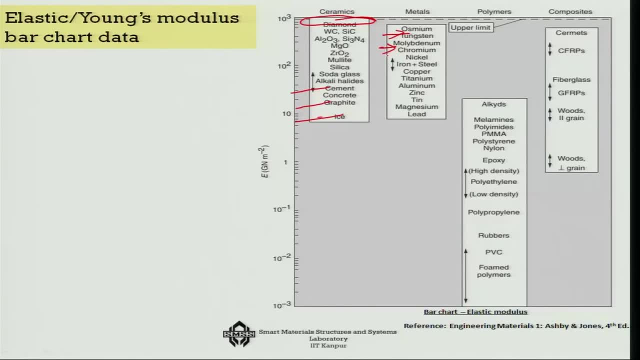 deform much less with the same application of force. And then where is the so? iron and steel is here, for example, 200 gigapascal kind of a thing. And then much softer ones are, for example, aluminum or zinc or tin magnesium. they are. 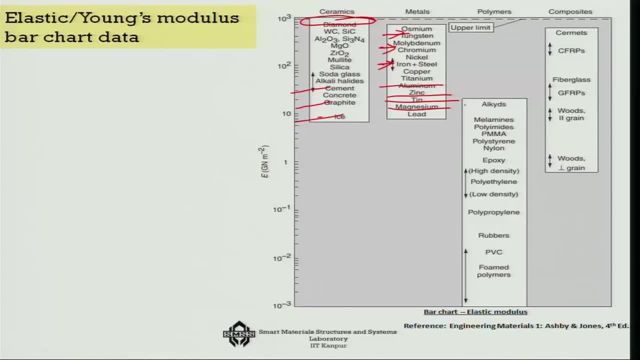 much softer in terms of the metals. So if you look at the polymers, you can see that there is nothing here That means the polymers are a degree, you know, several orders of magnitude lower in terms of the stiffness. 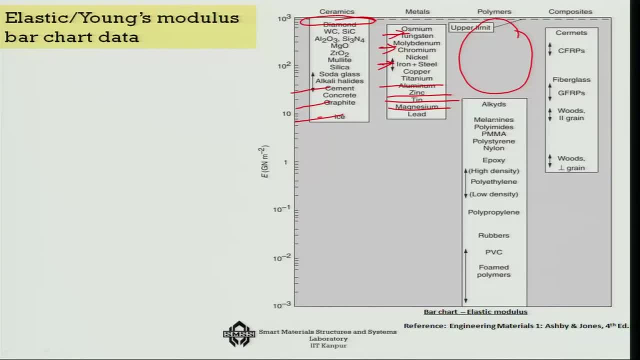 And there you know something like that is why I told you that about 2 gigapascal is something maximum that we generally observe, And there in the higher range, you get something like polymethylmethacrylate, polystyrene. 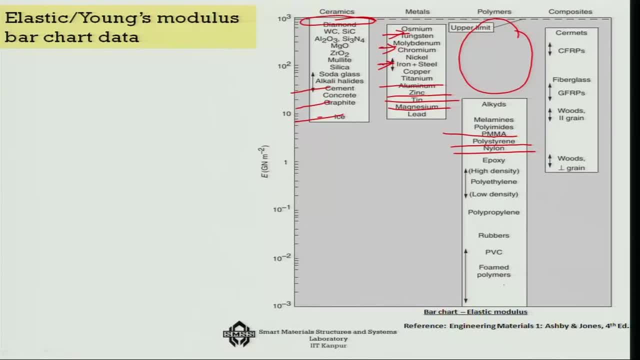 nylons, etcetera. And those which are very low are something like this, You know something like foamed polymers, PVC rubbers, etcetera. They show very low modulus of elasticity, or, in other words, the compliance is very high. 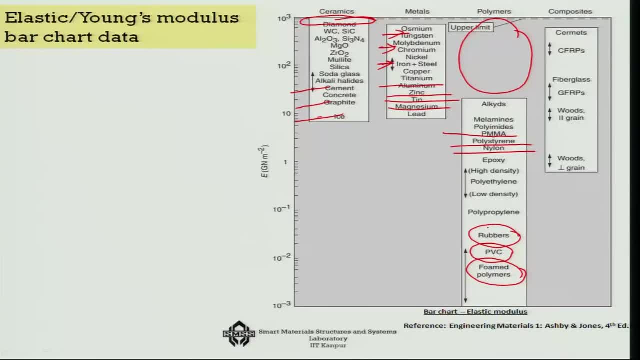 in such materials- Then if you look at the composites- composites, you know, the natural composites are generally softer, something like woods, etcetera, But the manmade synthetic composites actually have modulus of elasticity which is comparable. 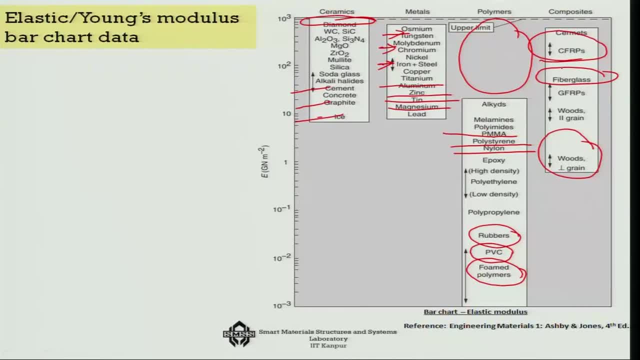 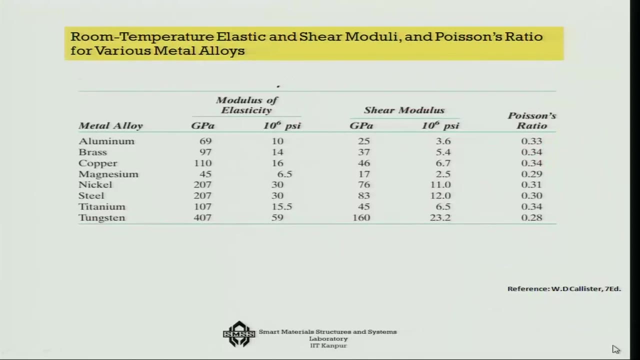 with the metals, fiber glasses, etcetera. So that is why composites are replacing the metals, you know, wherever the high stiffness is required. So that is, you know, kind of a comparison chart which you can, you know, keep in your mind. 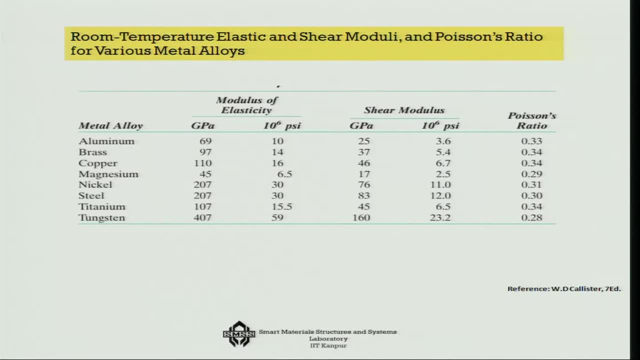 In terms of the absolute values. here you know, once again I have given three values we have given from Callister here And just for reference. for example, if you consider aluminum, approximately 70 gigapascal modulus of elasticity, shear modulus is approximately 25, and Poisson's ratio is approximately. 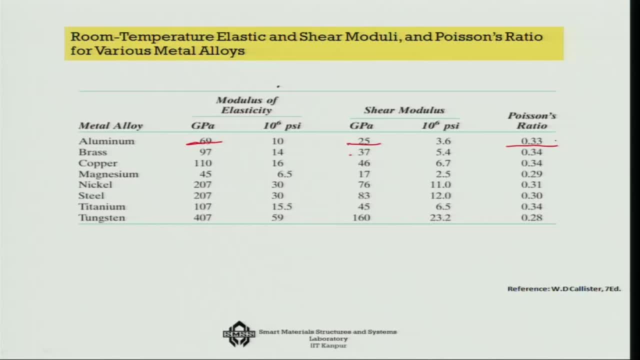 0.3.. So again in this list you would see that a high modulus of elasticity you are finding in something like tungsten And the shear modulus is also high in that same range, but shear modulus is usually 0.3.. 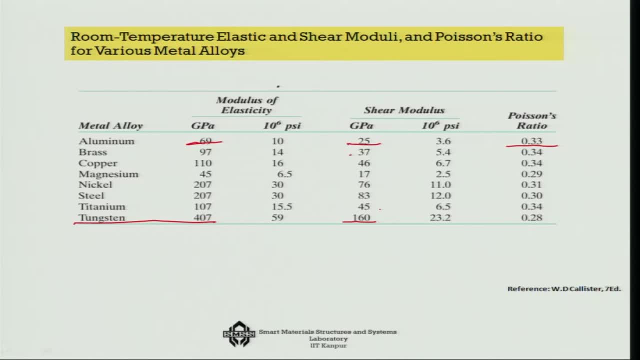 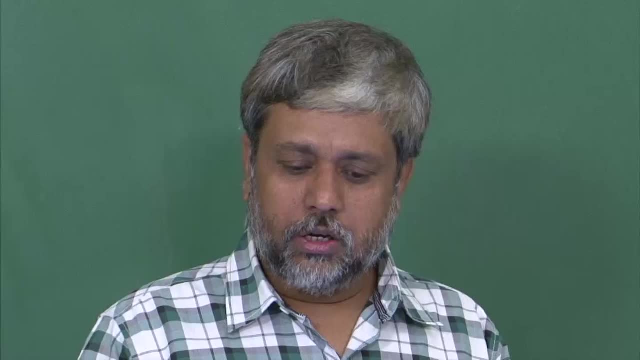 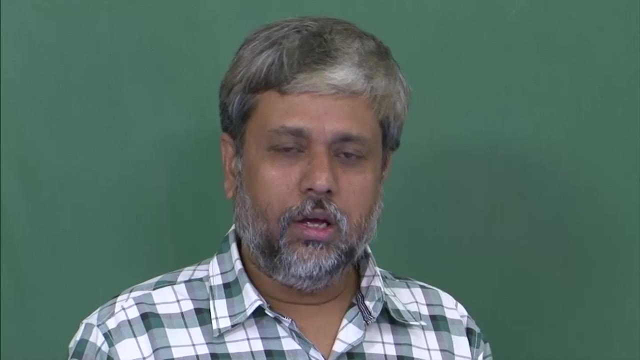 Similarly always lower in comparison to the you know Young's modulus of the system. What does it mean? It means that you know you can actually shear the material or twist the material, deform the material in the shearing mode much easily instead of actually 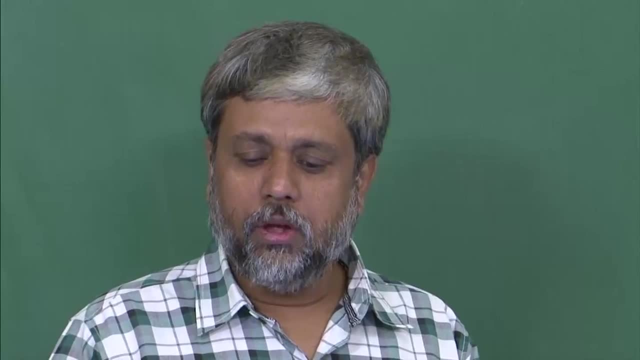 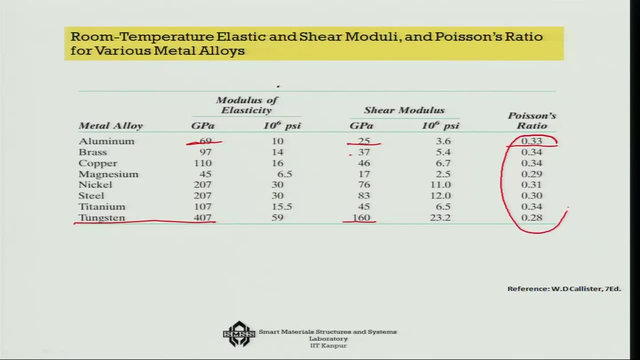 elongating or compressing the material And the Poisson's ratio, you can see, is not really varying. It is more or less in a range of, you know, 10 to 15 gigapascal. So this is a range of something like 0.3, around that range for most of the metals. So it is just 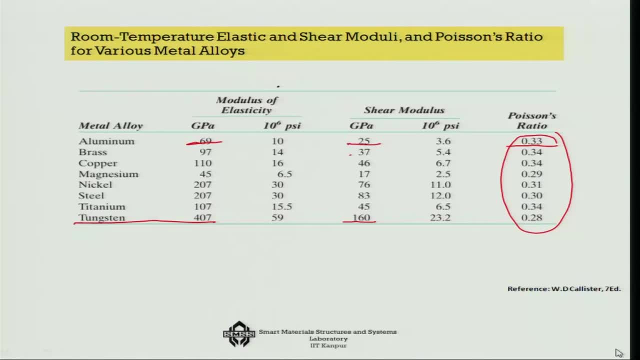 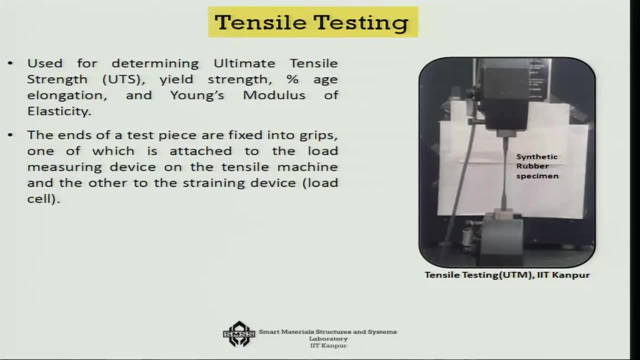 for a comparison of these properties in various metals. Now we carry out. you know how do we measure this property. In order to measure this property, we use a tensile testing system in a machine, which is known as actually, universal testing. 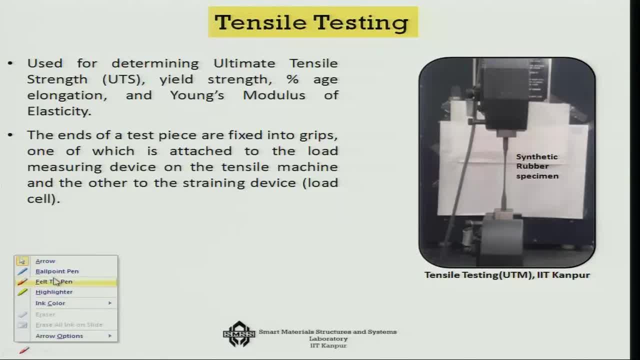 machine In which we find out properties like, for example, ultimate tensile strength, yield, strength, percentage elongation, Young's modulus of elasticity, etcetera. So I have just now shown you that in a UTM machine, how we are, you know, we can deform the rubber specimen. 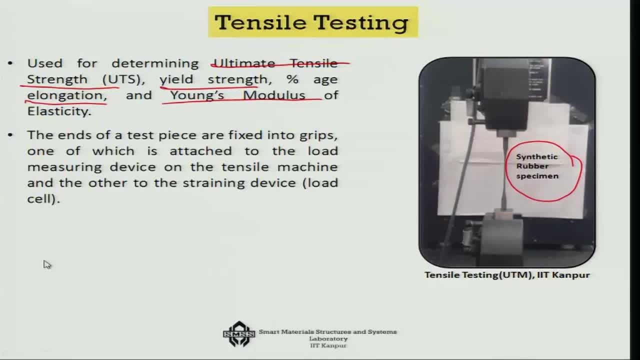 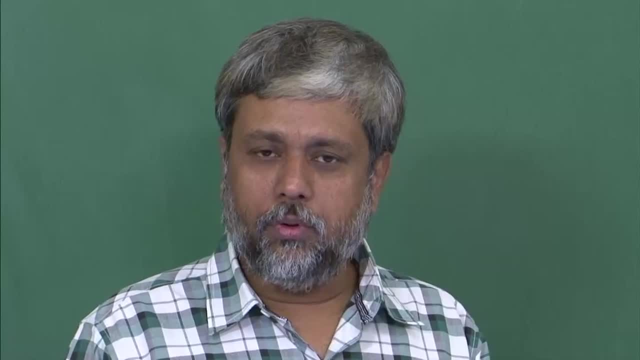 the same specimen that I have shown you can be used in this case. Universal testing machine is a beautiful machine where you can actually load a specific material. So you can actually load a sample in various ways: tension compression, shear, Not only. 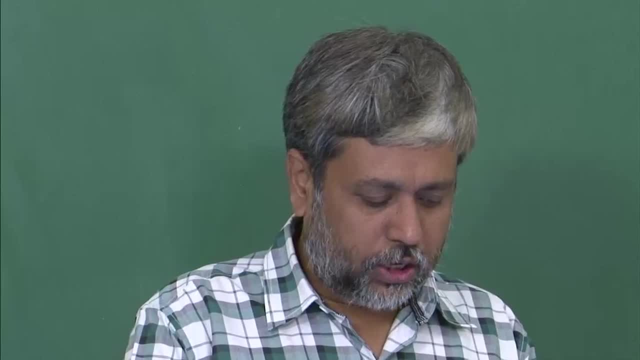 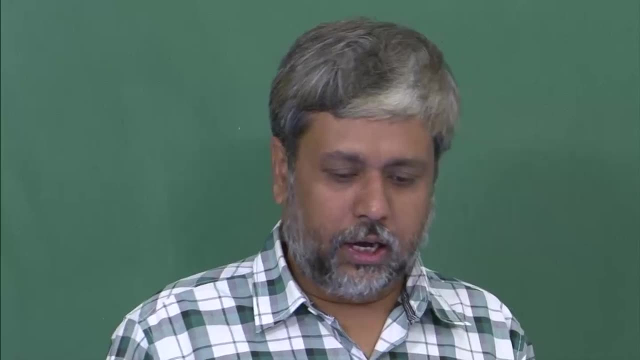 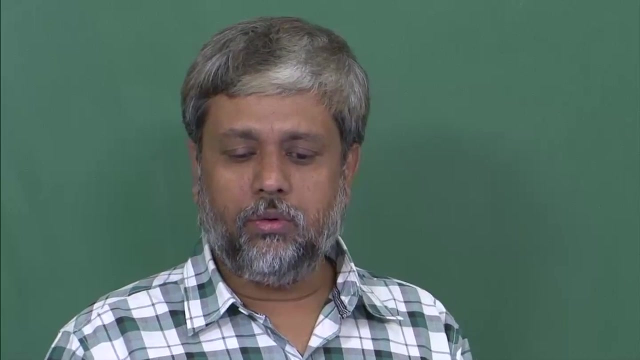 that the loading can be made dynamic loading and which can include things like fatigue, etcetera. So that is, you know how do we generally carry out this universal testing? you know, machine, the tensile testing. Now, if you carry out such testing of a ductile 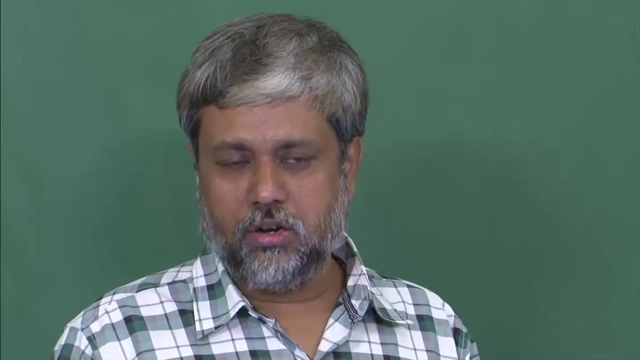 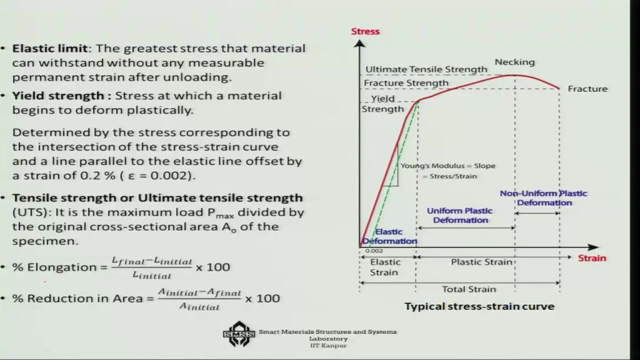 metal. how would you find out this tensile strength? How would you find out this stress strain diagram? And that is the, you know, the engineering stress strain diagram of the material. How do you usually see it? a stress strain diagram. 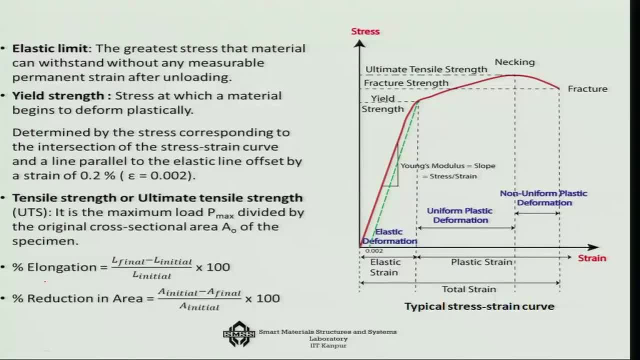 If you look at it, that the stress strain diagram shows certain features, But please keep in mind that this is for a ductile metal, So you will see that there is an initial region where you know the material. if 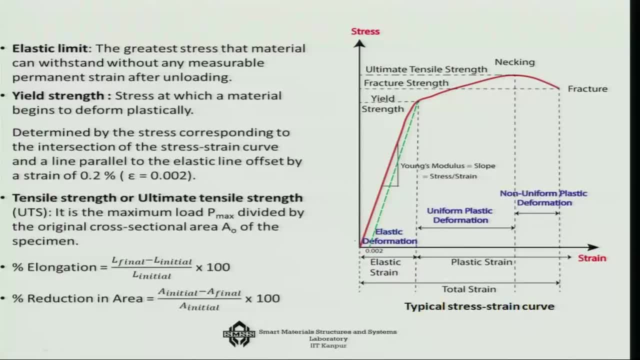 you actually understand the material, you can actually find out the stress strain diagram. So this is the stress strain diagram, So this is the stress strain diagram. And you know, if you unload the material it will come back to the same point itself And that 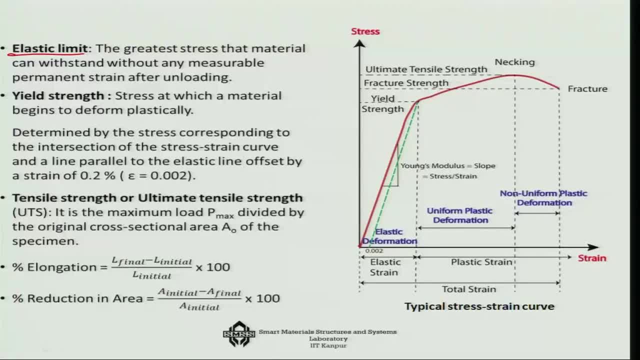 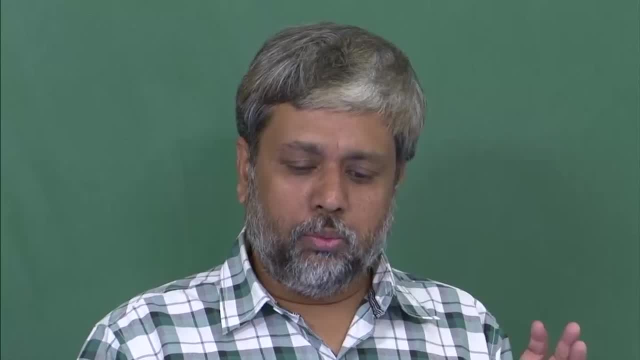 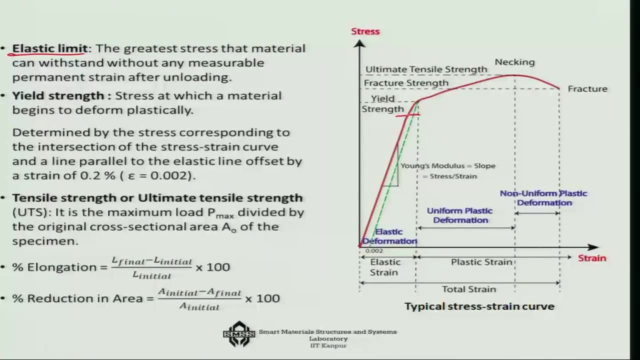 is known as the elastic limit. That means the maximum stress that can withstand without any measurable permanent strain after unloading. Now in the elastic limit, of course there are two regions In one region. up to some region it is actually perfectly linear, And beyond that it is slightly non-linear. But 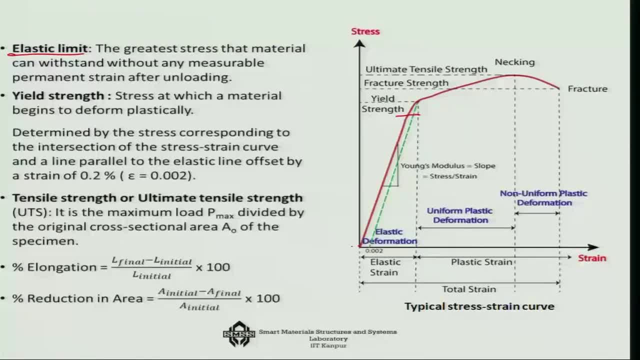 still, if you really is in the non-linear region, it will come back to its original orientation, And that is what is: the buildings in the elastic limit. Now then the point curves here, that is, the yield strength points Beyond the yield strength. 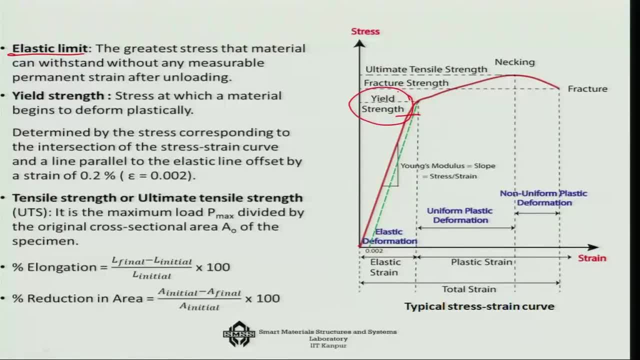 point, if you actually deform the material, then it will start to deform plastic. So what it means is that beyond that point, if you actually start to unload, there will be some amount of deformation which will always remain into this system, And that is why the 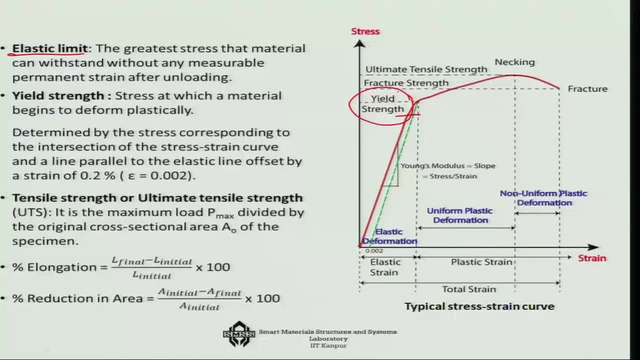 yield strength position is very important Because that sense of deformation starts to deform the material And that is the difference between the surface and the surface of the structure And that is why the yield strength equation of this diagram is very important. says the onslaught of actually plastic deformation in the system. 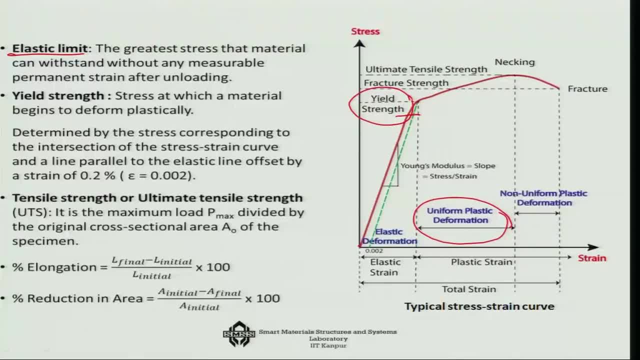 So, as I am increasing the load, I am going beyond the yield strength level and I am actually watching the uniform plastic deformation. Now, if I increase the load further, what is going to happen is something like a necking phenomena. that would start to happen and then the material will go to the fracture. 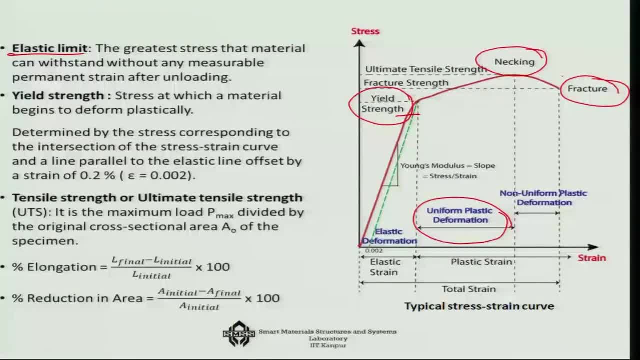 So that is what generally happens for a ductile material. So in that, beyond that necking point, what you get is a non-uniform plastic deformation. So the plastic strain itself can be divided into two parts. One is when it is uniform plastic deformation, that is the first part, and then when there 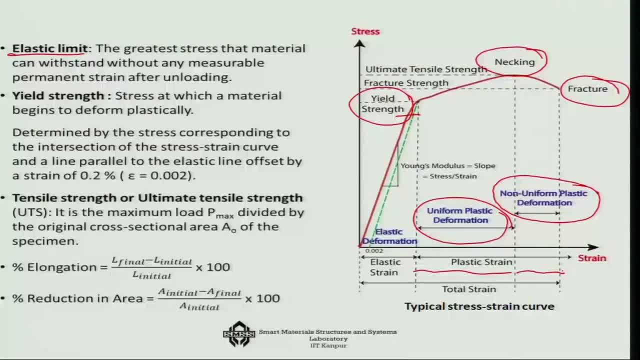 is a non-uniform plastic deformation till failure. So that is what we will find in the system, And what is the point? The point that is important for us is that up to the necking, we get actually the ultimate tensile strength. 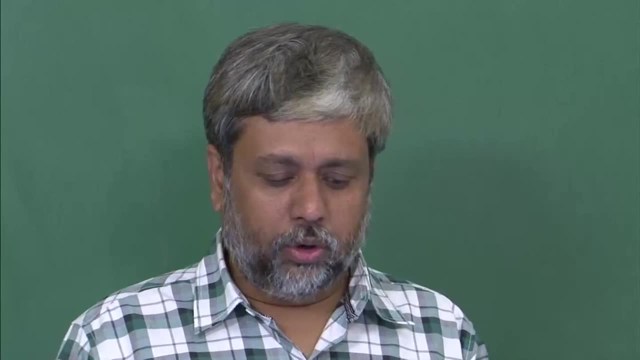 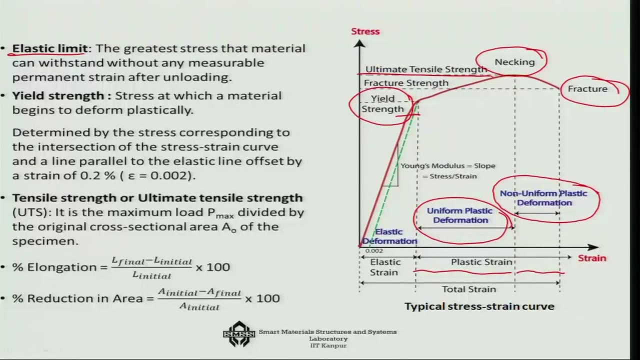 So that is the maximum load divided by the original cross-sectional area of the system. that gives us the ultimate tensile strength. Beyond that you would not expect a strength of the material, because beyond that if you take the force it is actually going to take us towards the fracture. 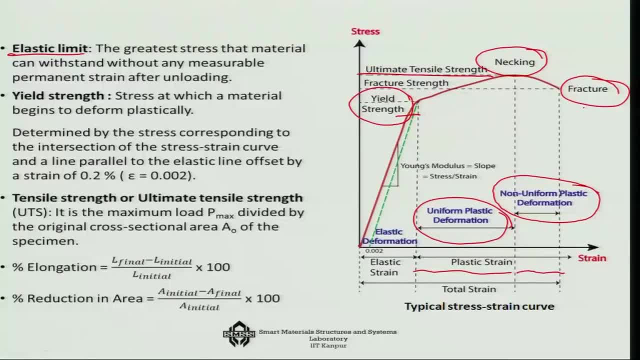 That is why ultimate tensile strength plays a very important role In terms of the product design And also the other two important factor is that: what is the percentage elongation, that is, the ratio of the difference of final to initial length change over the initial length? 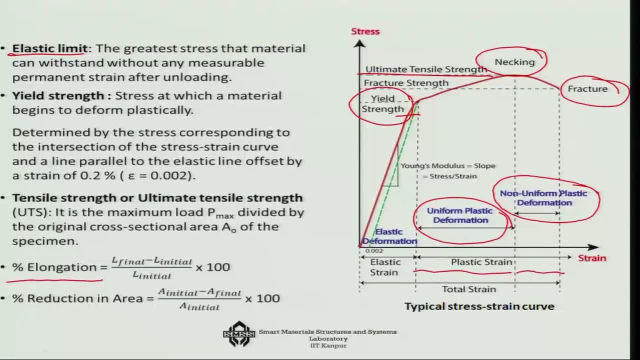 and similarly for the area. So that actually tells us that how compliant is the material. So this is a typical stress-strain curve for a ductile material. How will it look like for a brittle material? I can just vary the material. So this is a typical stress-strain curve for a ductile material. 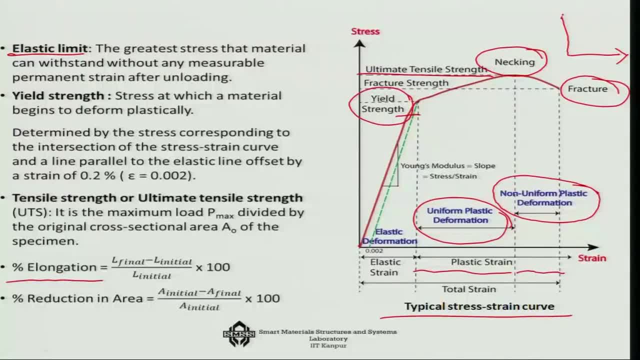 How will it look like for a brittle material? In a very small qualitative manner we can draw it here. that suppose this stress is denoted by sigma and strain by epsilon. So if I draw the sigma epsilon for a brittle material, it is just one single line and may. 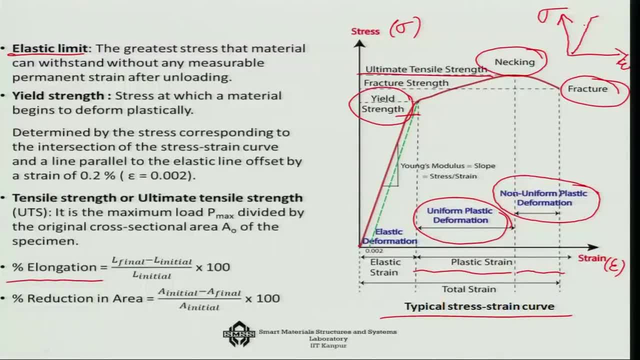 be some point of non-linearity, but that is it, and then it sharply fails. That means it will not show any plastic strain, any plastic deformation. That is generally happening. So this happens in terms of the brittle material. The other important point here is that generally the yield strength. if you do not find a very 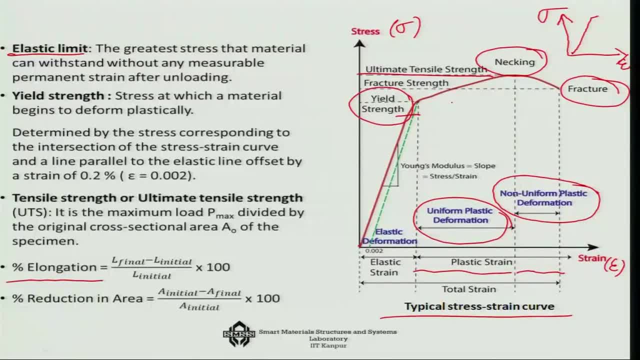 sharp point where there is, you know this is happening. we consider approximately this point: 0.002 level, That means the two percent strain level. we find out that where it is intersecting and that point is defined as the yield strength level, because that is generally the strain. 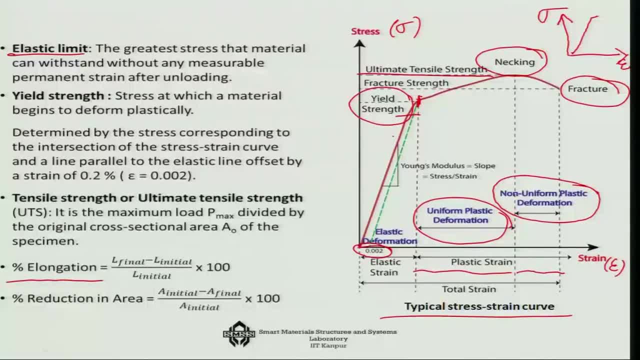 level which it can take in general. So the other тан asshole strain level we can reduce in metals without any permanent deformation, But this is very specific to the metals. For the things like elastomers or rubbers this can become something like 5 percent to. 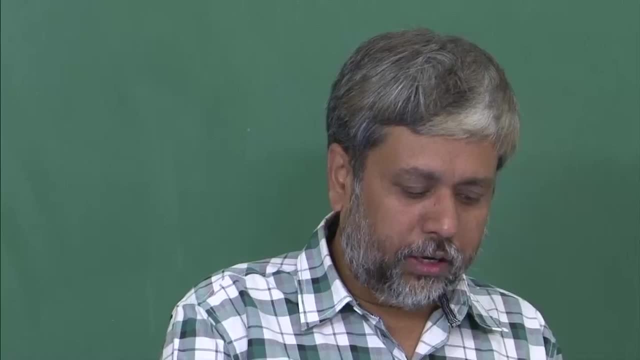 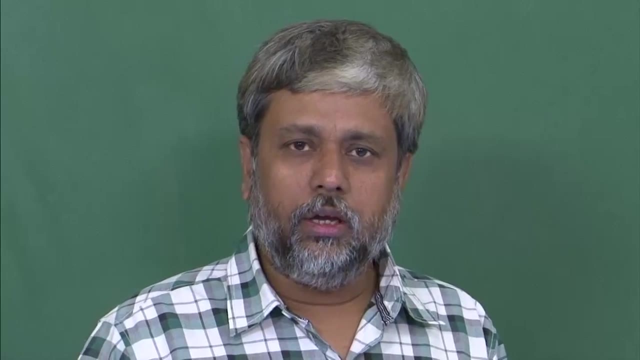 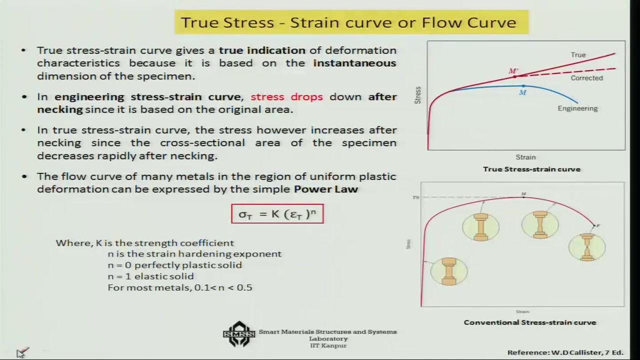 10 percent. So, depending on the material, this position may change. Now then, if we actually consider, however, the true stress-strain curve, that means if we consider that the area is actually changing, if you look at it, that as you are deforming, 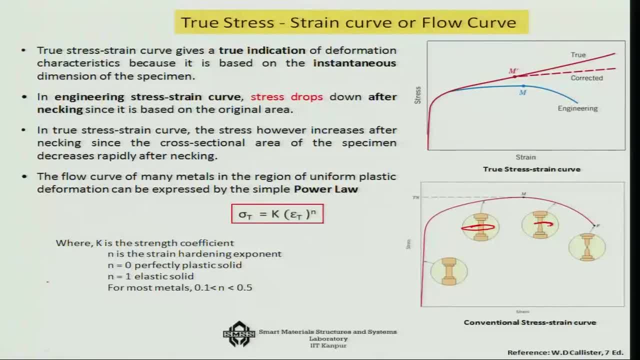 you know, this area is actually changing. This area is becoming smaller and smaller. The neck formation is happening. So the area is changing And if you consider that actual area, you will see that it is not actually. this stress-strain curve is not drooping. 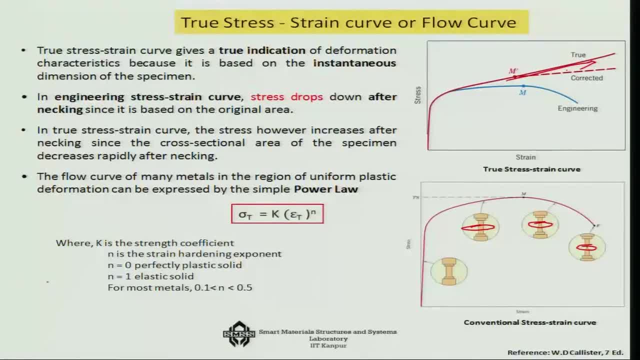 but it is actually increasing. And it is increasing because, even if the you know the force you are increasing, the force you are increasing, the area is actually decreasing at a very rapid rate. So that is why the you know the true stress actually is increasing at a very rapid rate. 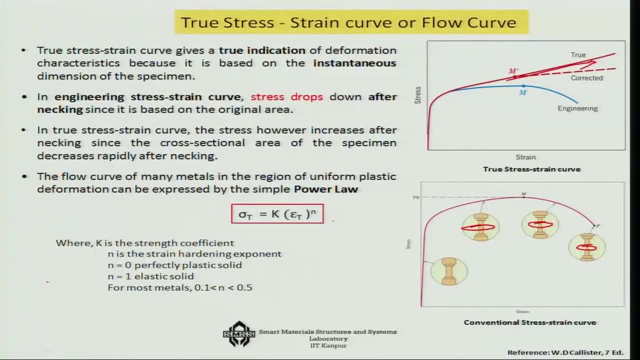 Now, in the uniform plastic deformation, this stress-strain relationship is actually governed by a power law which is like sigma t is k times epsilon t to the power n. where this n is 0 for perfectly plastic solid, n is 1 for elastic solid. 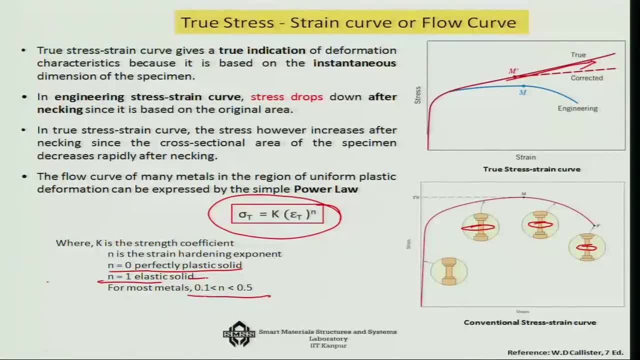 And for most metals it will be the plastic region between 0.1 to 0.5.. So that is how it would behave, you know, in the true stress-strain curve, which we generally overlook. Actually, we only look at the stress-strain curve that comes after the UTM machine. So 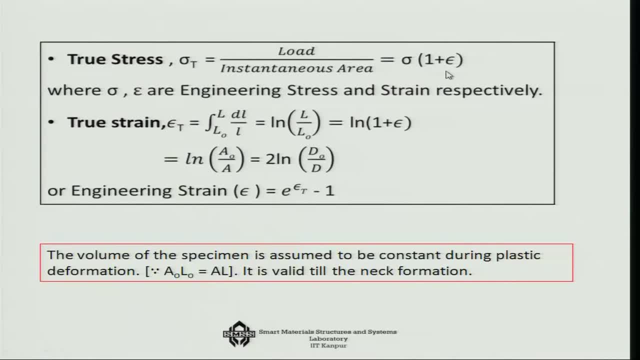 the true stress-strain curve. actually, true stress is denoted by this relationship, which is something like: what is the p everywhere p square? p square is equal to 1 by 2 over something like the sigma t as sigma times 1 plus epsilon and the true strain epsilon. 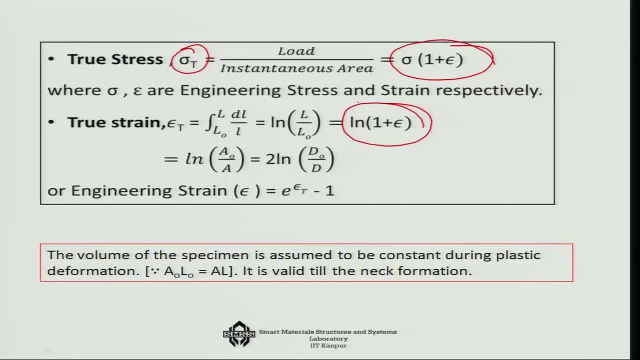 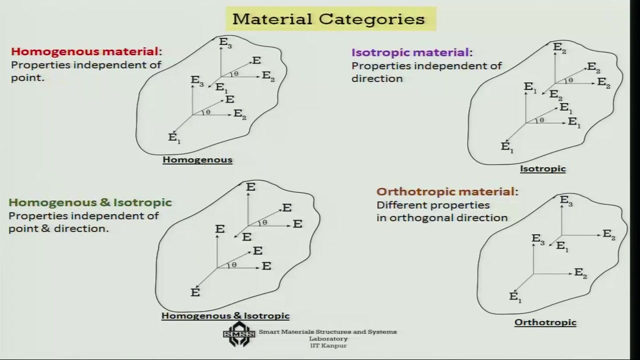 t is log of 1 plus epsilon, And the relationship between engineering strain and true strain is governed by this relationship. So this is what you can, just very simply, you know, mathematically you can actually obtain this relationship. Now, the other point is that the materials based on these stress relationships are actually 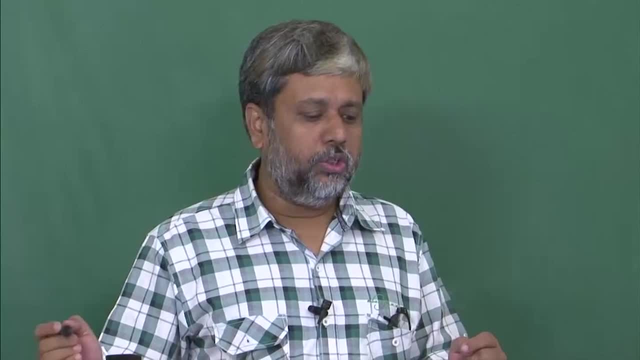 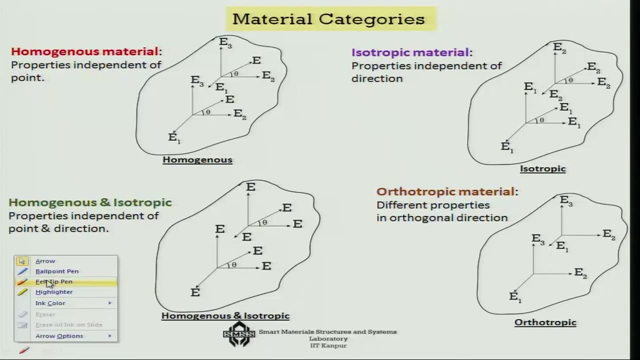 divided into sub, sub categories, like the homogeneous materials, for which the properties are actually independent of where I am measuring the property. That means: here you get a property and here you get a property, the all the directions. if you look at it, you are going to find the 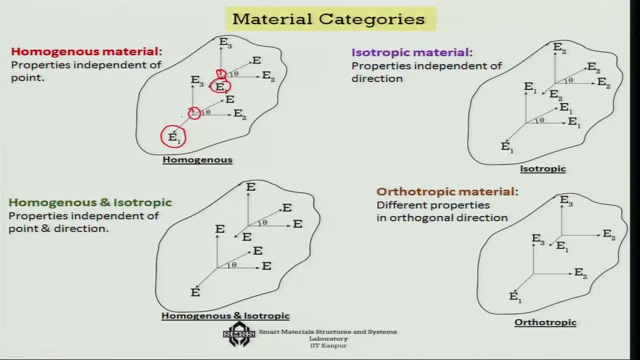 same modulus of elasticity, but it varies from direction to direction. So this is what you can, just very simply. you know, mathematically it is different to direction. In one direction it is E 1, in another direction it is E 2.. So 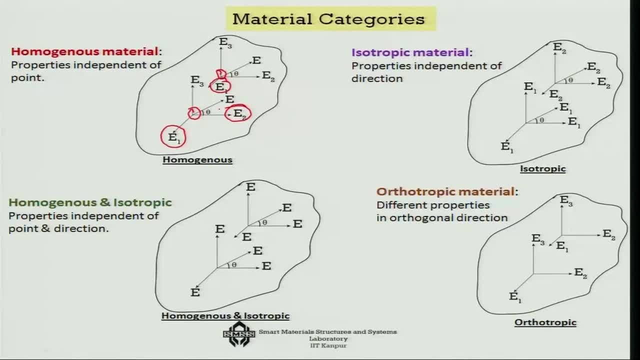 that is what is a homogeneous material, Whereas different points, you get the same pattern of modulus of elasticity. For isotropic it is actually direction independent. You get this, you know, at a particular point. if you consider you get E 1 in all the directions. 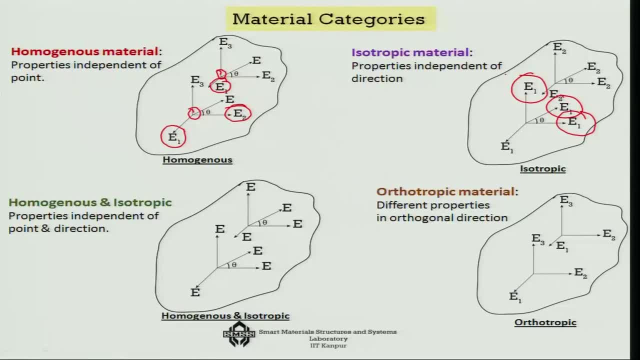 but if it is not homogeneous, then at a different point you get E 2 in all the directions and E 1 and E 2 are not the same, not the same. If they are same, then they will become a homogeneous and isotropic material. 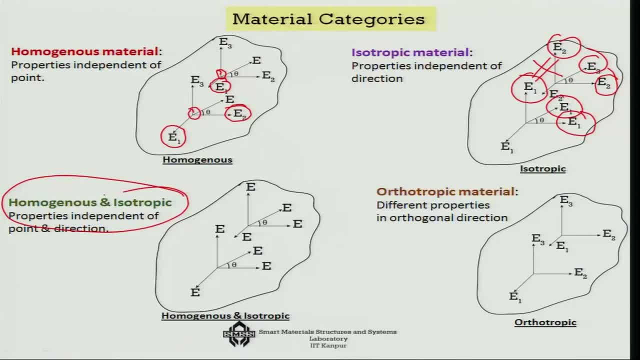 And if we consider an orthotropic material, in that case it is slightly different. In that case you will see that at different points it is homogeneous, but the modulus of elasticity varies in different directions, In the sense it varies in three different. 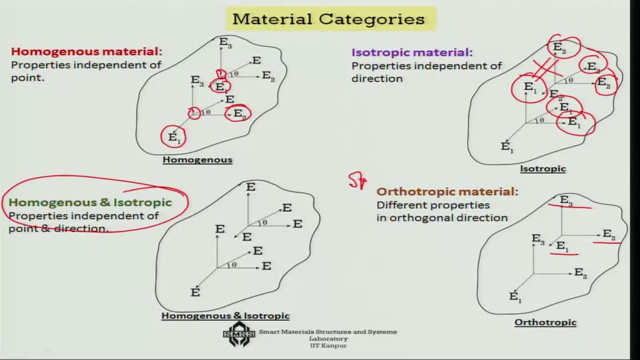 mutually orthogonal directions, that will be U 1, E 2 and E 3.. This is for generic, you know, general orthotropic material. but for spatially orthotropic material, you know, you may disregard one of them and it only varies in one set. That means something like: 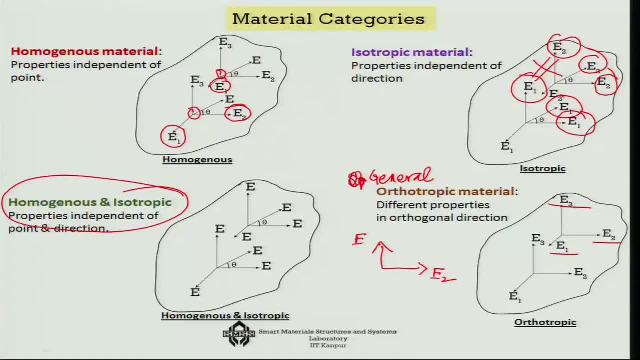 E 2 and E 3 will vary, but U 1 may remain the same. So that is what happens for spatially orthotropic material. This is typically a case like if you consider a laminated composite, then each lamina which 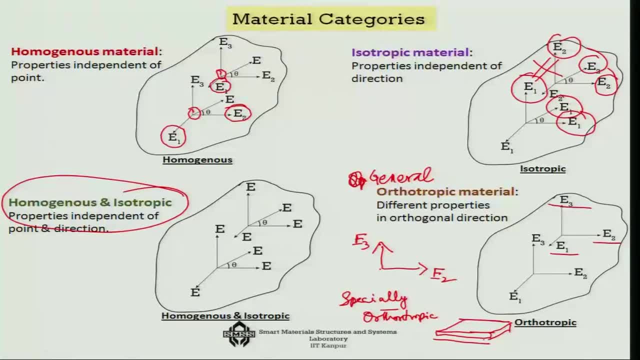 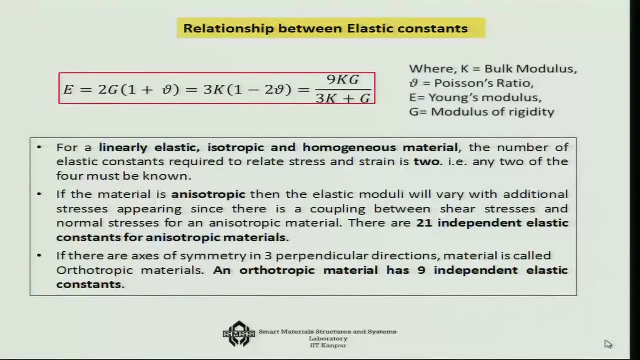 is very thin in one direction are actually considered to be spatially orthotropic material. So that is a very special case of a general orthotropic material. Now, the relationship, this elastic constants are actually related to each other by the relationship which 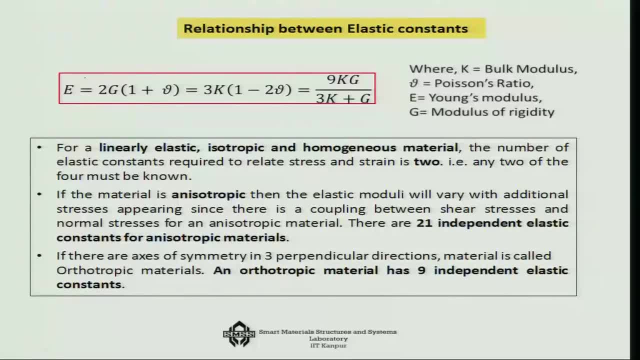 is shown here that the E is related to G and G is related to K. Hence, if you know, for a linearly elastic, isotropic and homogeneous material you need only two elastic constants and then the other two. That means we have these four. 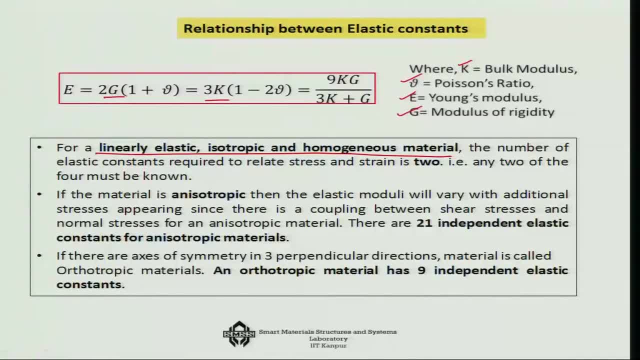 K, mu, mu, e and g. out of them any two. if you give me, i should be able to derive the other two, provided the material is linearly elastic, isotropic and homogeneous material. however, in case of anisotropic material, there are twenty one independent elastic constants. ok. 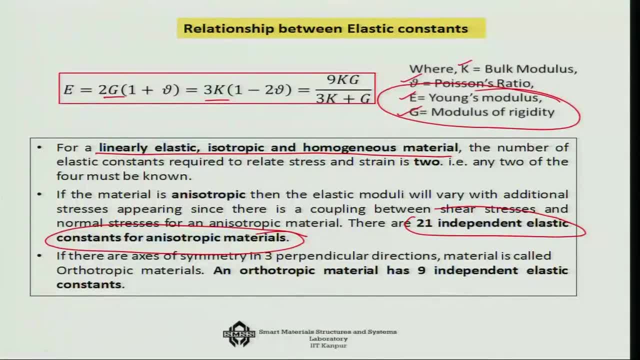 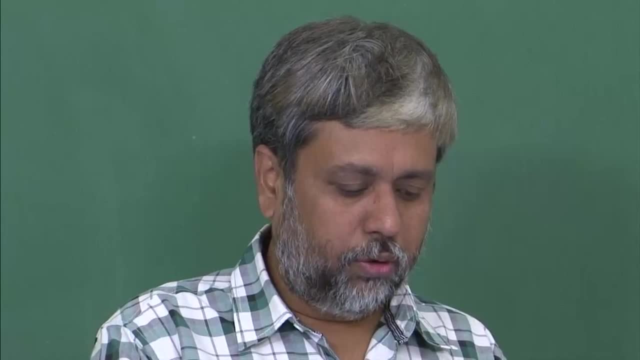 so it is a much, much higher, you know, in terms of the variations. and if it is orthotropic material, then it has nine independent elastic constants that will come into the picture. so naturally the tailoring is much more for an orthotropic material. now, that is the relationship. 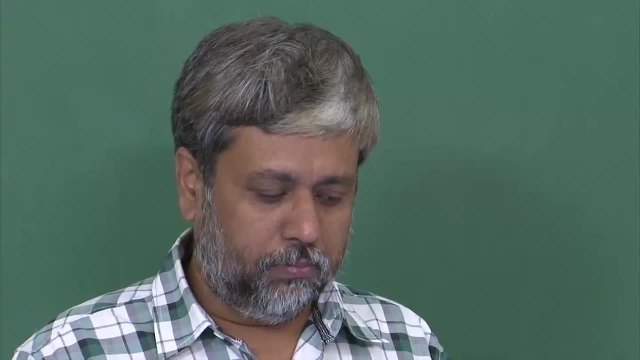 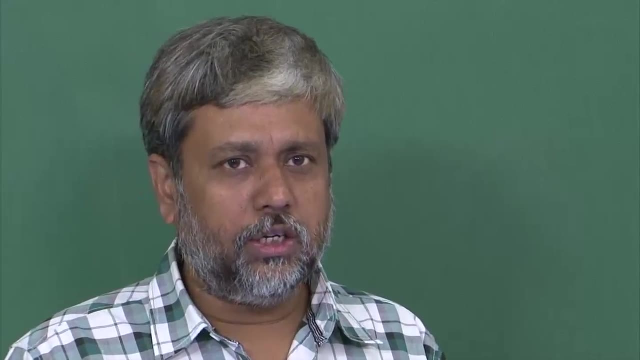 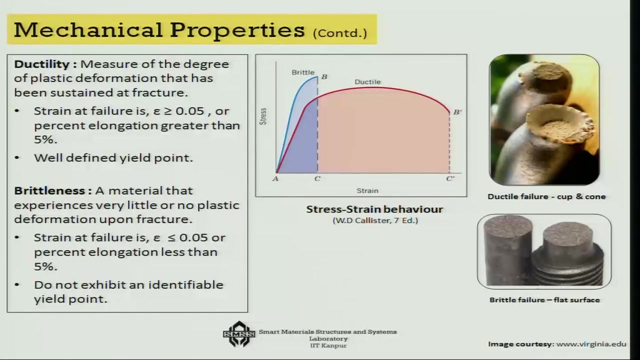 you know, in terms of the, actually the isotropic and orthotropic and anisotropic materials, the, so that is about the stress-strain relationship. there are some other mechanical properties which are also there. One of them is ductility. I already talked about it, that you know. it is the how much. 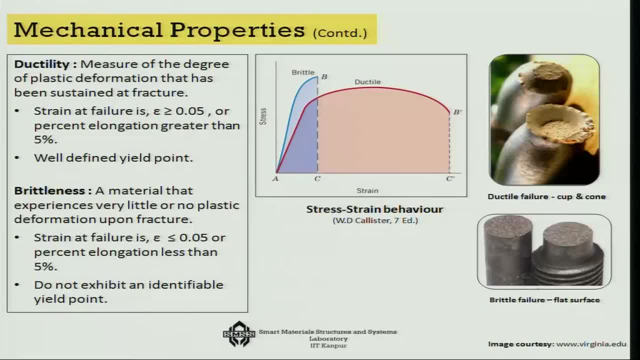 you know, is the capacity of how much you can draw a material under the tensile stress. ok, and that is very important. and there is something that you will also see in terms of ductility, which is known as the ductile failure, the telltale sign of the neck formation of the 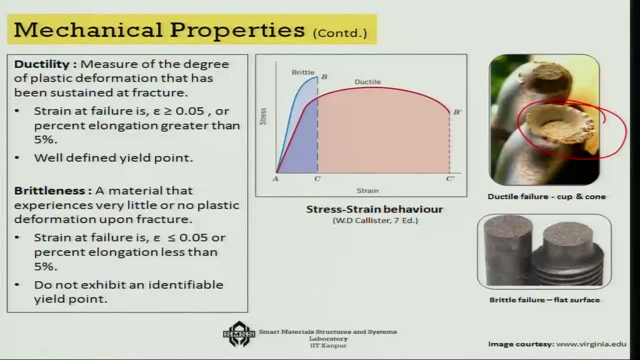 system and the brittleness of a system, The difference between a brittle and a ductile system. I have already drawn this stress-strain card for a, you know, brittle system and a ductile system. is that precise this ray? you know the presents of this plastic strain that is there for a ductile material and that is absent. 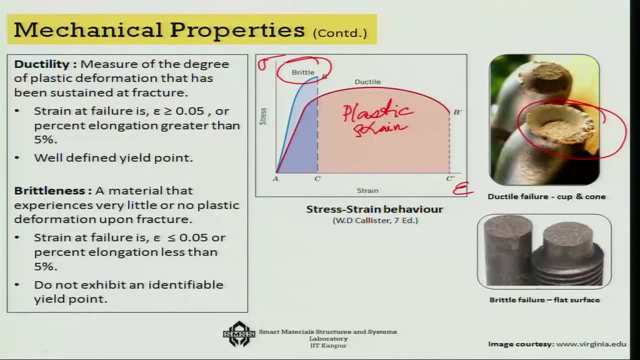 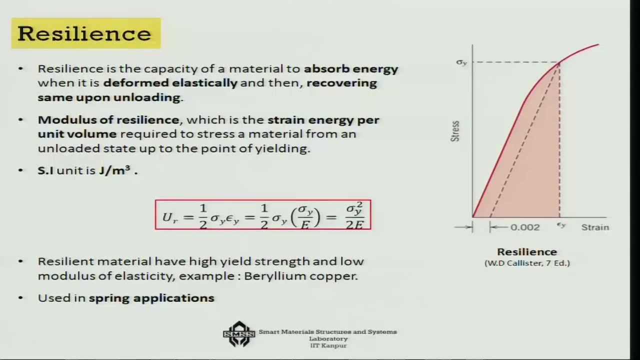 for a brittle material. So that is very important point that we have to keep in our mind while comparing between various material. Now, this is the real difference between a brittle and ductile. Ok, Thank you very much. material properties. Now, the other important point here is actually the resilience of a 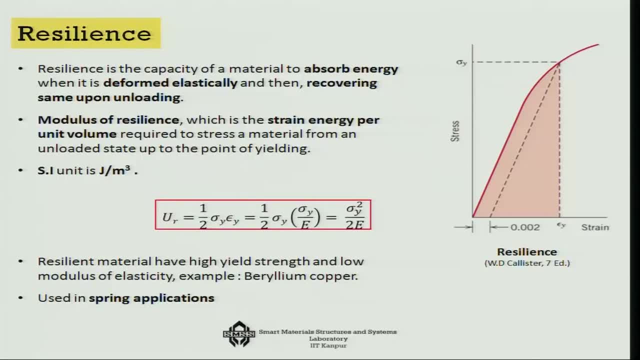 material, which is the capacity of a material to absorb the energy elastically. So it is in the elastic domain When it is deformed elastically. how much of energy you can absorb. If you consider the stress-strain diagram and if you consider the area under the stress-strain, 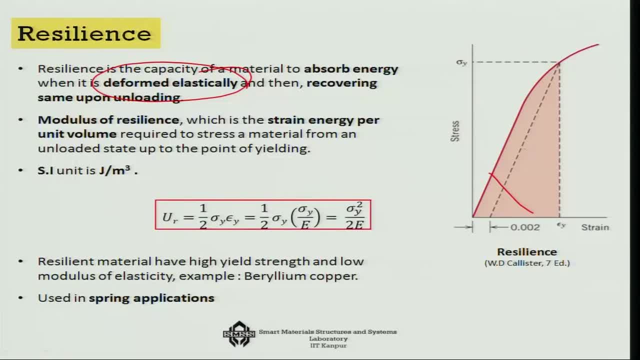 diagram you can actually find out that this is something like you know sigma y square over 2 e in a kind of an approximate measure. And that is so. that means, if you know what is the yield stress and if you know what is the modulus of elasticity, you can actually 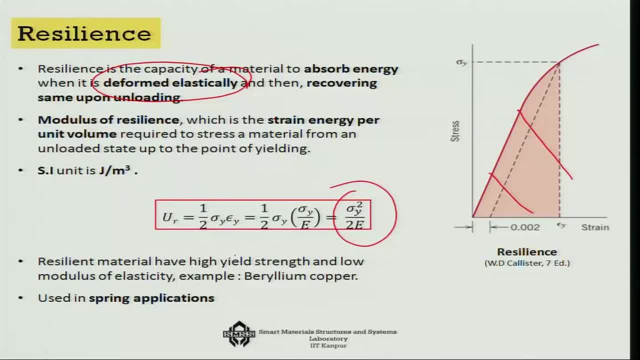 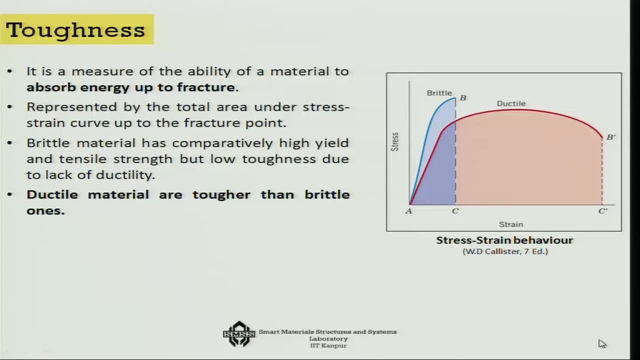 compute that. what is the resilience of the material in terms of modulus of resilience and how much of energy the material can absorb, which is very important in applications like spring type of applications. So the resilience is another important mechanical property. The last important property in this direction is the toughness. Toughness is also the area 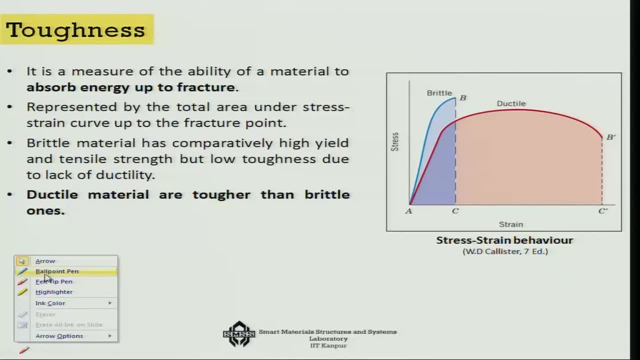 under the stress-strain curve, just like the earlier, you know, in this case, But here you are considering the plastic region also. So earlier you were confining yourself within the elastic region, Now you are considering the plastic region also. In fact, the test. 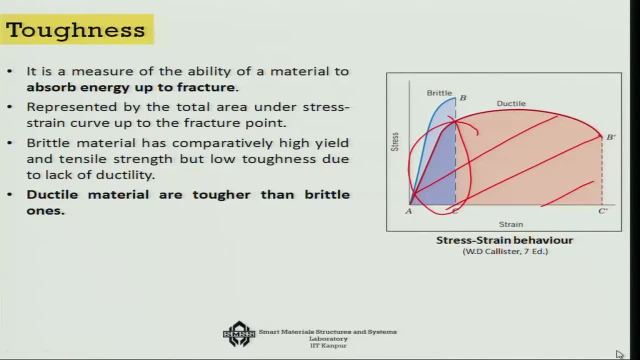 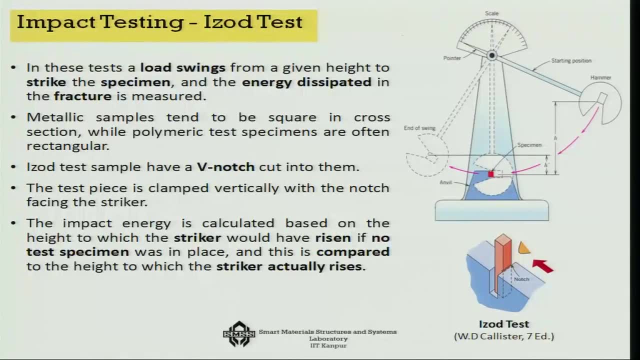 that is very important is that if you consider the area under the stress-strain curve, you are considering the elastic region also. So the test that is very much important towards this direction are actually Izod and Charpy impact test. So this is an Izod impact test where actually you support the sample from. 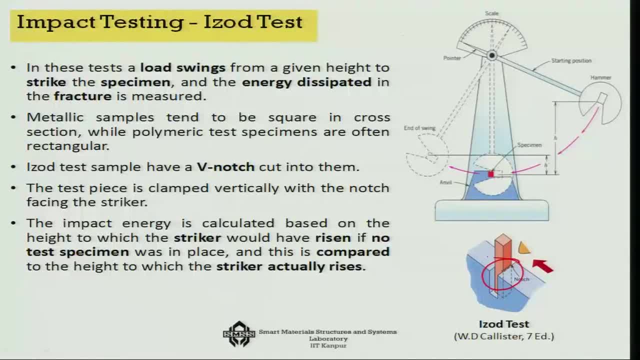 one position here: You are supporting the sample and you are hitting it through a pendulum, And if there is no sample, then it can go to a particular distance. If there is a sample there, then some energy is actually taken by it, So it cannot go. you know up to that. 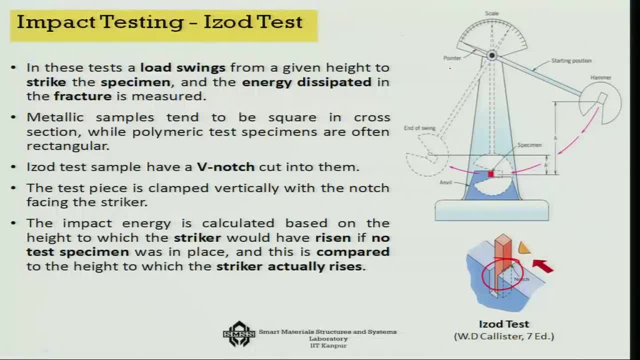 distance. So you take that ratio of the two, the return ratio, you call it, and then that gives a measure of how much of energy is actually absorbed by the material, and which is a measure of the toughness of the material. Now, similarly, there is another very similar test actually, which is known as the Charpy. 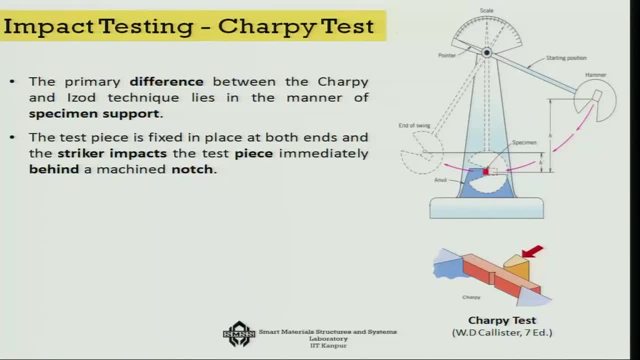 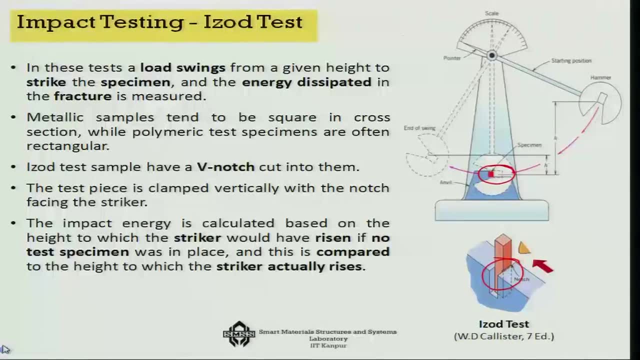 test. Now, the difference between the two tests, the Izod test and the Charpy test, is that in the Izod test you have… You have, you know, for example, if I go to the last case, you have the crack which? 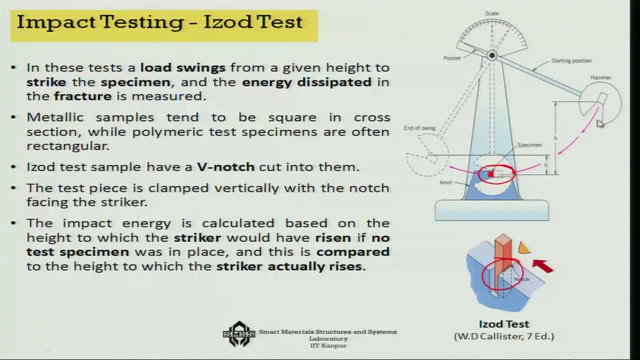 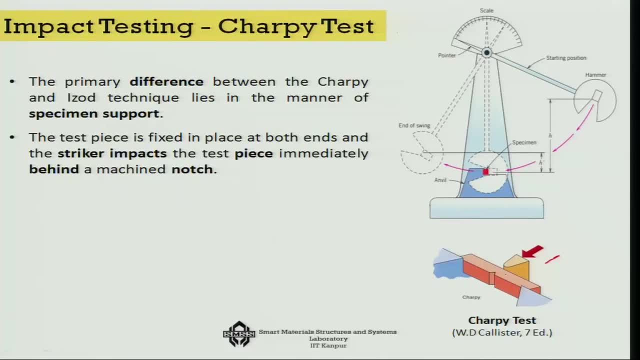 is you make a notch actually, and the notch actually faces the hammer, So the hammer faces the notch, you know. So you are in terms of Charpy, as you can see. on the other hand, the notch is at the opposite side of the hammer, So that is one of the difference. 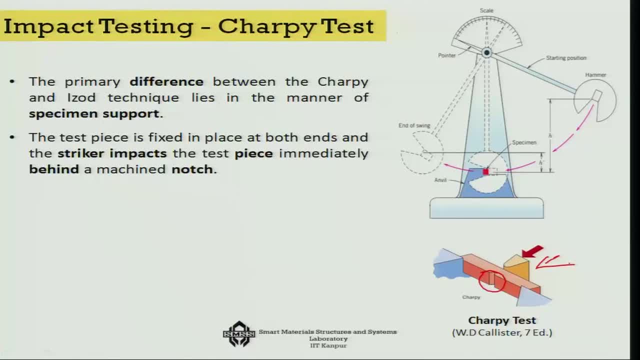 between the two, You know, And also in case of a Charpy test, you are supporting the material at two places instead of at one location. But both of them are very good tests which can measure that, how much of energy a material can absorb, and that means how tough the 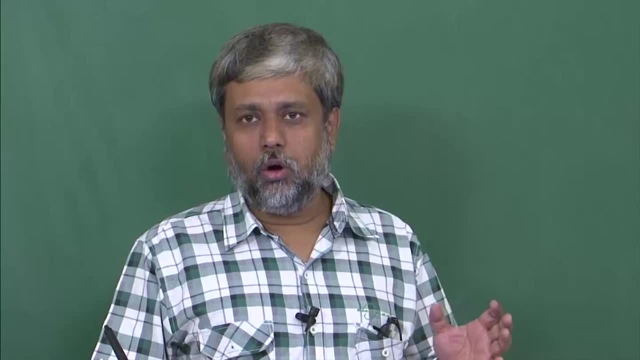 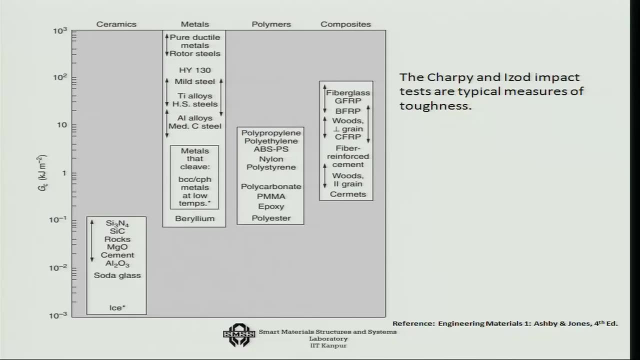 material is and that actually means that you know how much is the impact strength that is there in the material. So here is, you know, some kind of a comparison of a from the as we stable and as you can see here, if you look at it very closely, that the metals are. 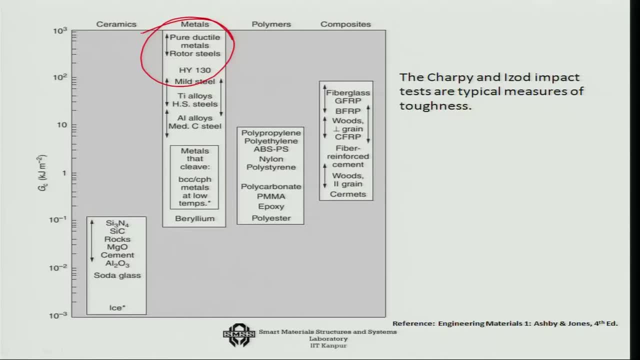 stopping in the least, actually because they can absorb quite a good amount of impact energy and in fact, plastics, even though the deformed mode, they cannot absorb that much of energy. brittle materials, of course, are the worst here. So that is what is in terms of the 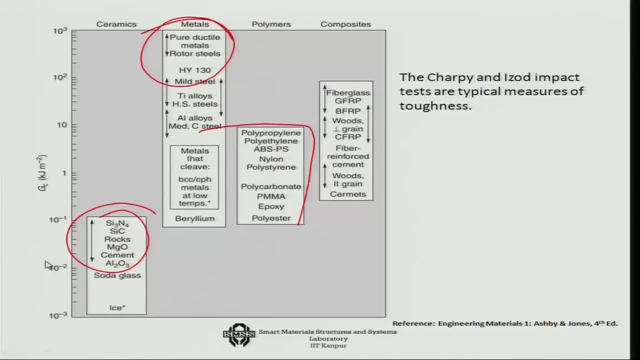 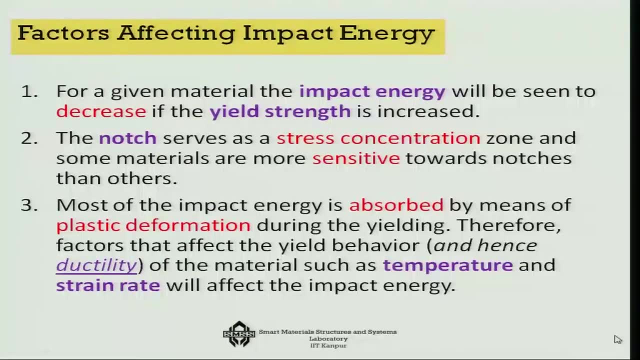 three different, you know, groups of materials, and composites are somewhere in between. Now the factors that are important in terms of the impact energy is that for a given material, you know the impact energy will decrease if the yield strength is increased. So that is generally found in a material and the notch serves as a stress concentration zone. So 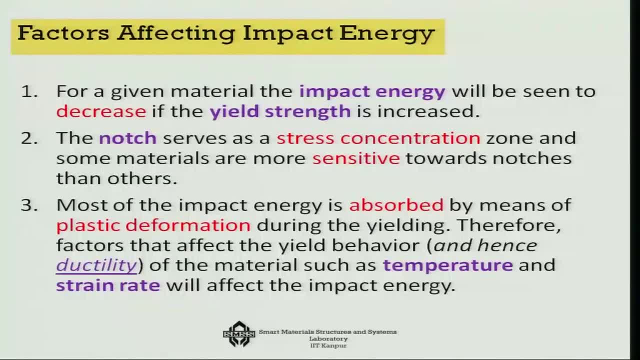 some materials are more sensitive to notches and the most of the impact energy is actually absorbed during the plastic deformation of the material. also, temperature and ductility plays a very important role on it. So this is where we are going to close this lecture, and in the next lecture we will discuss about the material. So that is all, Thank.